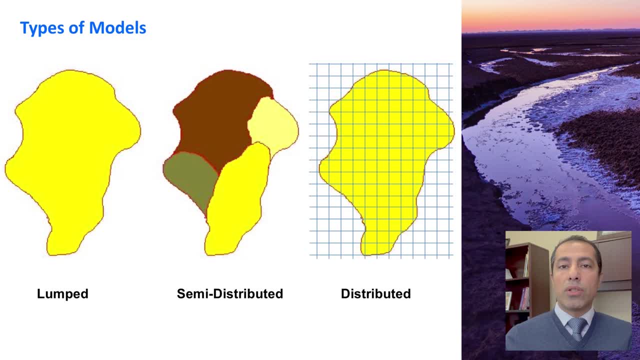 typically a gridded model with regular or irregular grids and in each grid we calculate all the processes in our model. Obviously, distributed models are more complex, they require more data and they only make sense if we have the required spatial information. From model structure viewpoint, we have 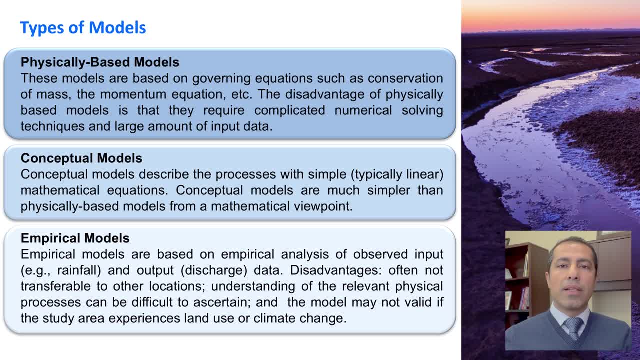 broadly three types of models: physically based, conceptual and empirical. Physically based models are based on governing equations such as conservation of mass, the momentum equation and so forth. They typically require a lot of data and, of course, numerical modeling. Empirical models: 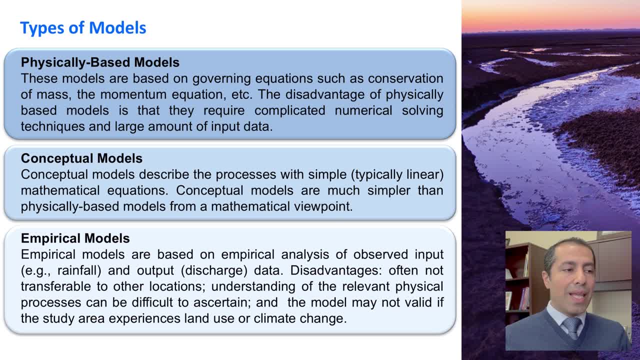 on the other hand, are very simple and based on empirical observations, such as rainfall and river discharge data. There are many useful empirical models in the literature, but they have some limitations. Often they are not transferable from one location to another. They cannot be used to describe. 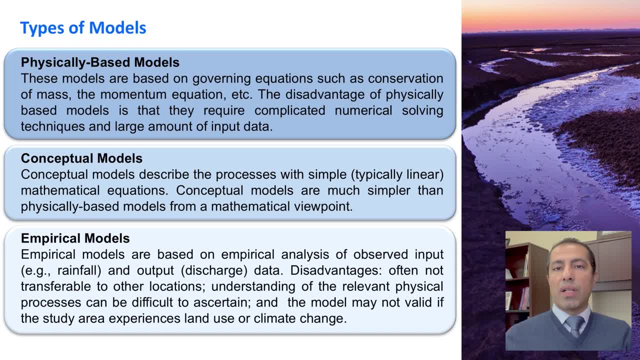 changes in land use, land cover or climate conditions. Also, we can't use them to really understand physical processes and interactions between different variables. Conceptual models describe the processes using simple mathematical results such as numbers, values and so on. Conceptual models provide the process to control a lot of different variables, such as real air and wind, global warming, global warming of air conditions and climate conditions. Using simple mathematical models, we add a whole range of variables to the model. For example, even a large and complex model might be enough to know the usual data of individual properties. 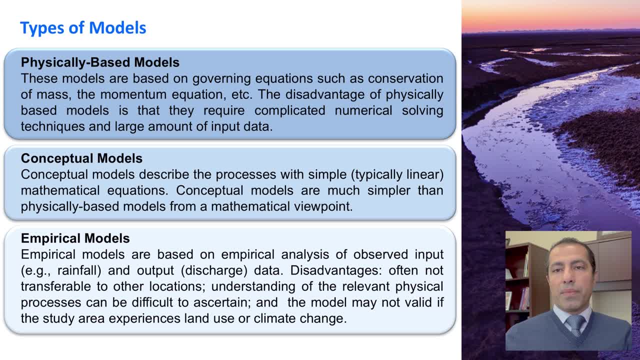 We can't use them to really understand the physical processes and interactions between different variables. Conceptual models describe the processes with simple mathematical examples, functions, typically linear. They are much simpler than physically based models, more complex than empirical models. Many of our widely used hydrologic models are 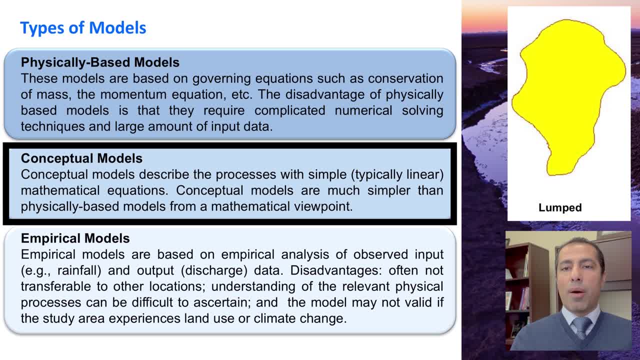 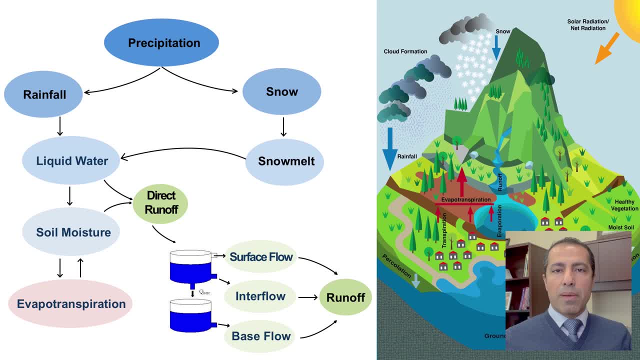 conceptual. In this lecture we develop a lumped conceptual model. This is our model structure. We start with precipitation, we decompose it to rainfall and snow, we calculate snowmelt and liquid water and other relevant variables like soil moisture and evapotranspiration to calculate runoff. 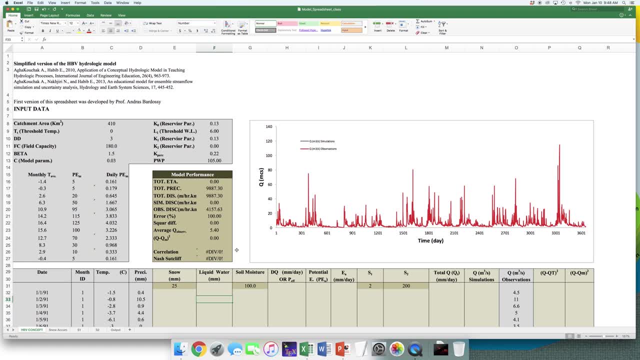 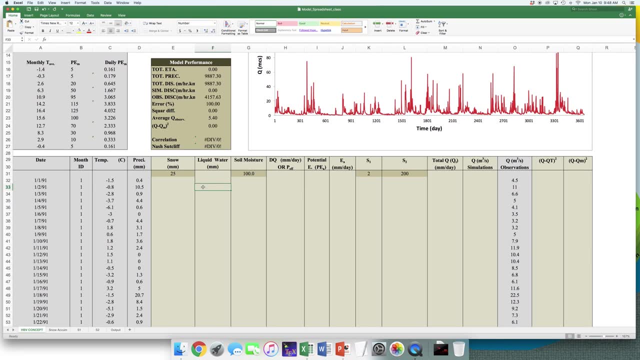 This is the model that we will develop together. Again, we use an Excel spreadsheet, start with some input data and we develop the model step by step. Download this Excel spreadsheet from my website and follow all the steps with me. Here we have an example of a model that we will develop together. We start with: 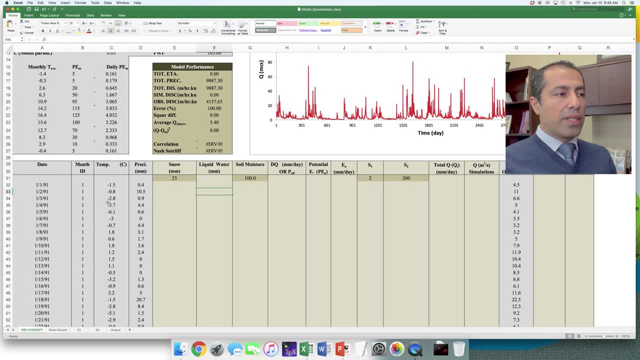 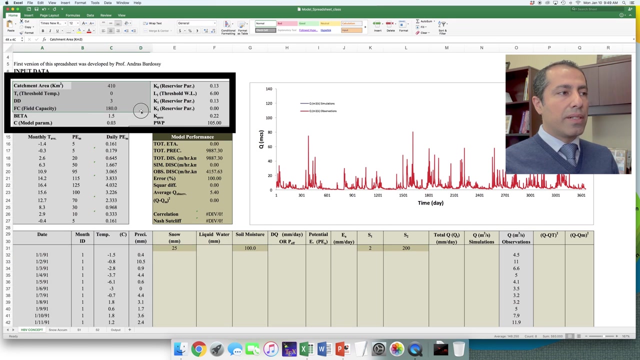 10 years of data. one vector of temperature data: daily temperature. each day we have one single value and precipitation in millimeter. Here our input data are in gray columns, so our main inputs are temperature, precipitation and observed discharge. We also have model parameters, and as we go, 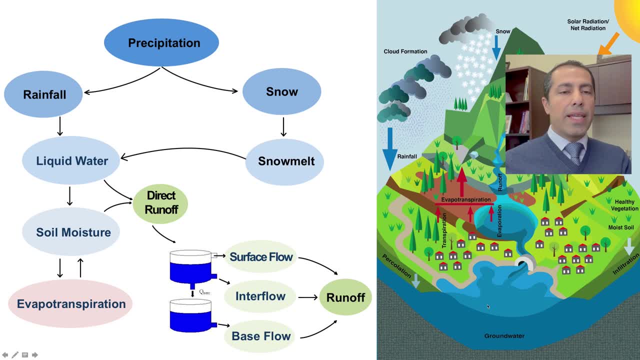 through. I'll introduce model parameters Again here. I assume that you already have some background in hydrology, so I do not focus on describing methods for evapotranspiration or soil moisture estimation. Instead, I focus how we link these processes. Of course, in each part I will briefly 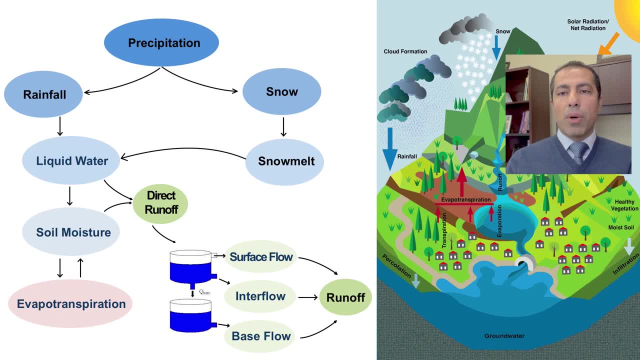 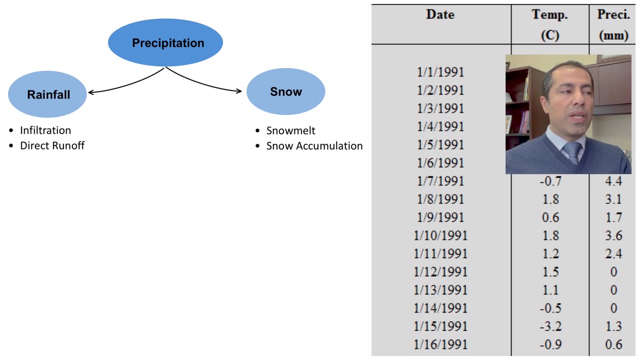 introduce one single method for hydrologic modeling. but I do not cover fundamentals of hydrology. My main focus is on modeling. The first step in our model, flowchart, is decomposing precipitation to rainfall and snow. because we want to make some simplifying assumptions. We want to assume that if 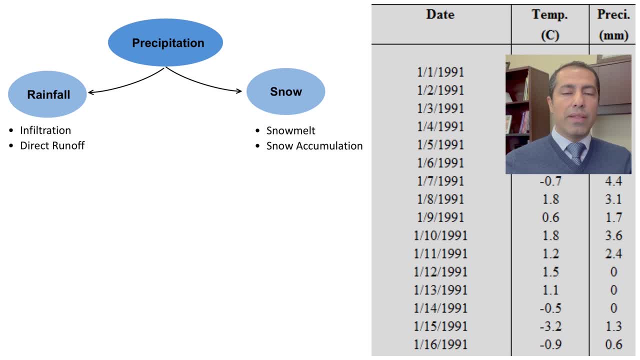 precipitation falls in form of snow. we won't have infiltration or direct runoff. It means precipitation does not translate to runoff immediately. It comes down in form of snow and it remains there until it melts. It's a strong assumption We know. in reality it does not necessarily. 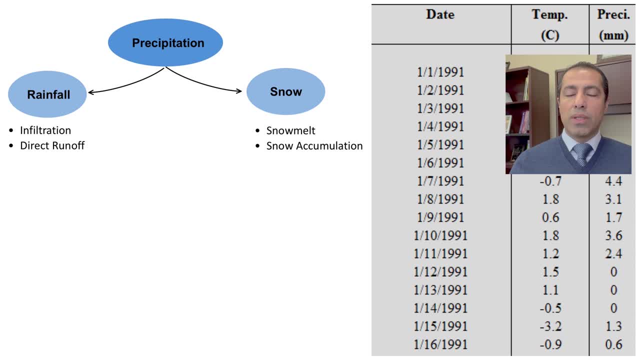 like that. but we have to make some simplifying assumption to model rainfall runoff processes. If rainfall occurs or precipitation in liquid form, we have to calculate infiltration and direct runoff. It means some of that rainfall will infiltrate and some of that will immediately turn into runoff. 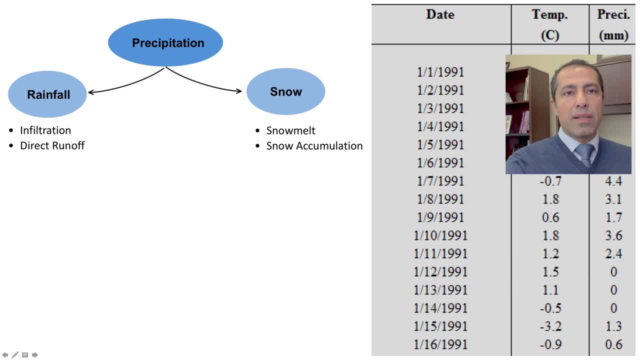 In our Excel spreadsheet we have 10 years of precipitation, daily precipitation and temperature data. We have to make an assumption for decomposing precipitation to rainfall and snow. One very common assumption is: if temperature is below or equal freezing level, we assume the entire precipitation falls in form of snow, and if temperature is above, then the entire. 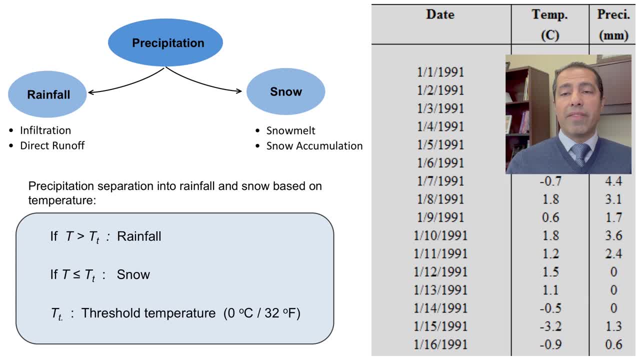 precipitation falls in form of rainfall. This is a very strong assumption. We know in reality that when we make a decision on precipitation or freezing, the whole system falls into. We can have rainfall below freezing level or snow above freezing level, especially because sometimes there is a big difference between air temperature close to the surface. 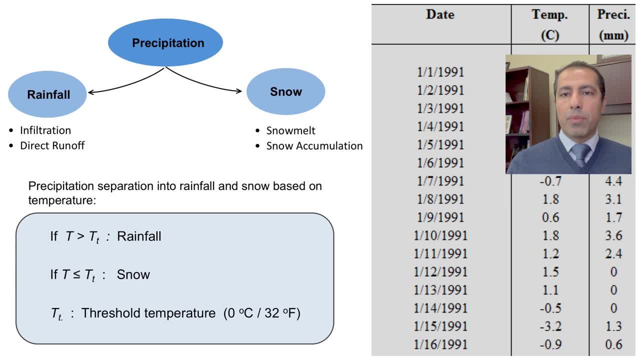 and air temperature high in the atmosphere that dominates rain versus snow formation. We know it's a strong assumption, but it allows us to simply decompose precipitation into rainfall and snow. We call the freezing level our temperature threshold, or TT. We assume temperature threshold to be 0 Celsius or 32 Fahrenheit. 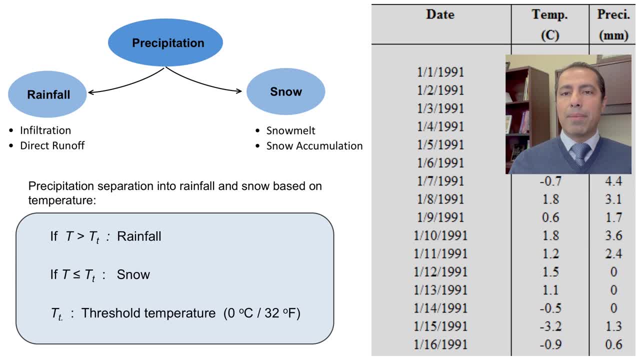 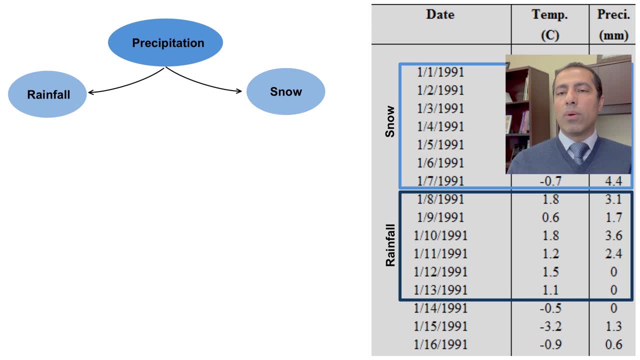 and we can revisit our assumption when we get to parameter estimation and calibration In our Excel spreadsheet. the first seven days temperature is below zero, So we assume the entire precipitation falls in form of snow and the next day's rainfall occurs When snow occurs. 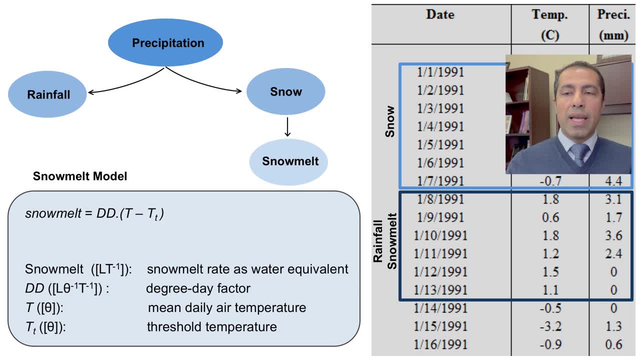 we have to keep track of snow, calculate snow accumulation and also snow melt. Here again we make a relatively strong assumption. We assume if temperature remains below zero there is no snow melt, And when temperature goes above our temperature threshold- freezing level in this case- snow melt starts. 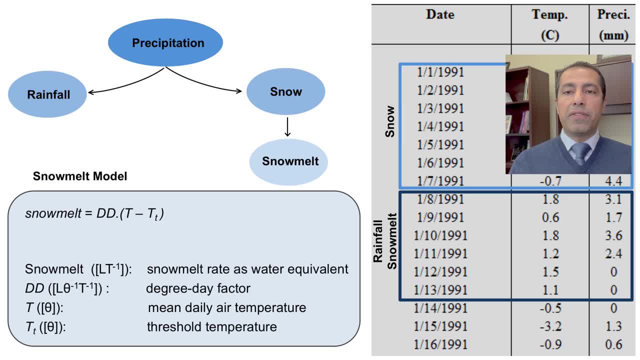 This is a strong assumption, especially when we are close to freezing level. We know that, in reality, even when the temperature is below zero, snow melt occurs. But this simplifying assumption allows us to easily calculate snow melt. Here we use a model based on degree day factor. 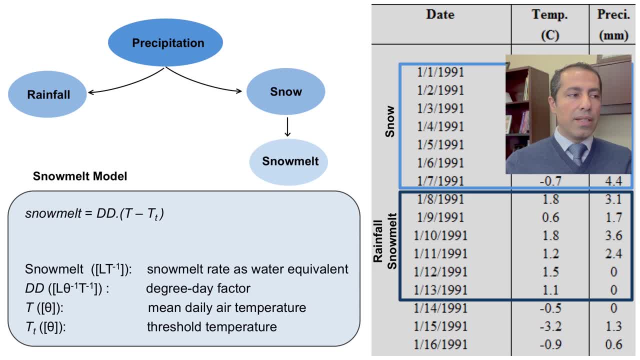 Snow melt is equal to degree day DD times temperature. that's daily temperature T minus our fixed temperature threshold. Temperature threshold in this case is zero Celsius. Degree day describes how much snow can melt per degree per day. For example, if degree day factor is five millimeter per degree per day. 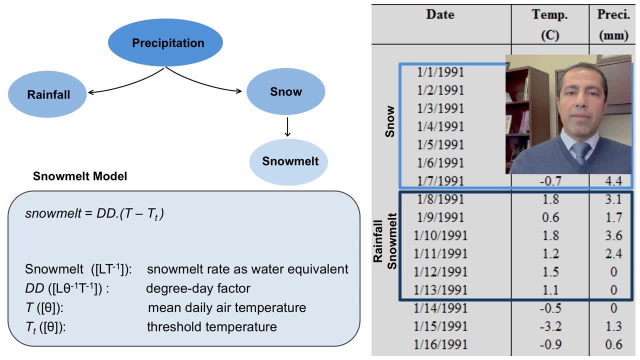 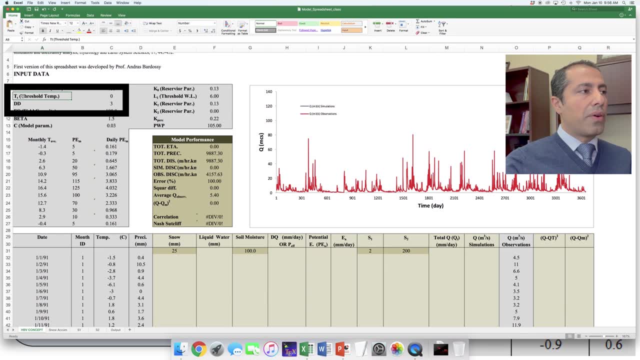 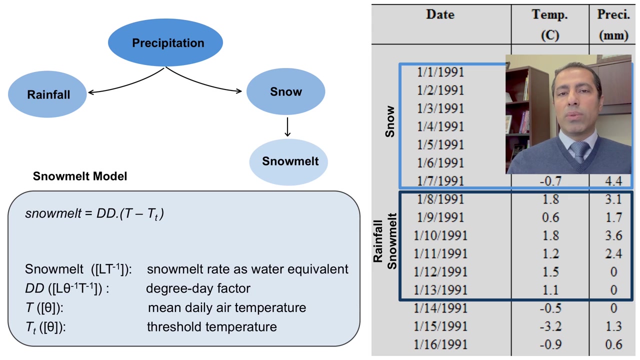 it means for every one degree deviation from freezing level, then five millimeter of snow will melt per day. In our Excel spreadsheet, temperature threshold here is zero And our degree day factor is three. How to estimate degree day factor? It can actually be measured, but if you don't have direct data, 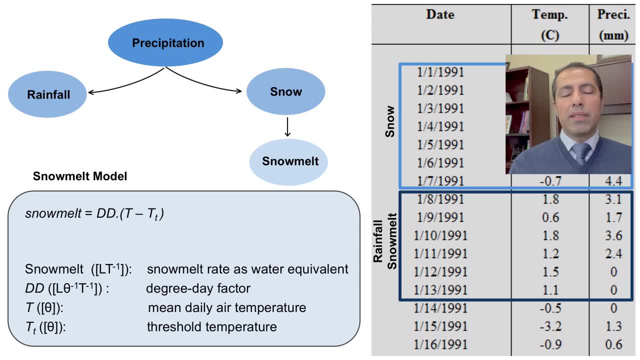 you can either look into other similar studies in the same area, published papers and reports, or simply make an assumption first, And then later we will learn how to revisit and evaluate our assumption. In our Excel spreadsheet we also have an initial value for snow. 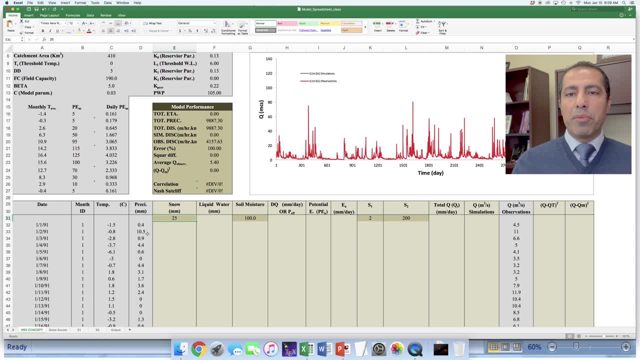 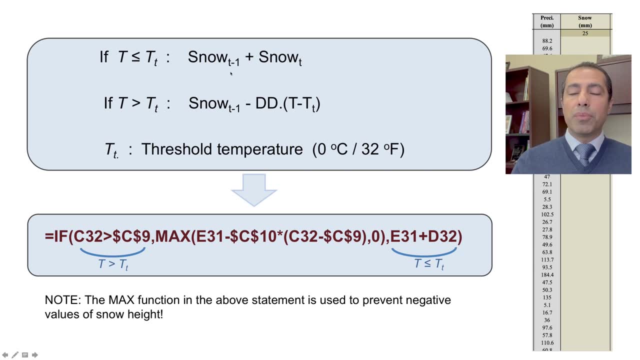 It is 25.. It means there is 25 millimeter of snow already on the ground. before we start modeling Again to calculate snow, we have to keep track of snow accumulation from day to day and also calculate snow melt when temperature exceeds zero. 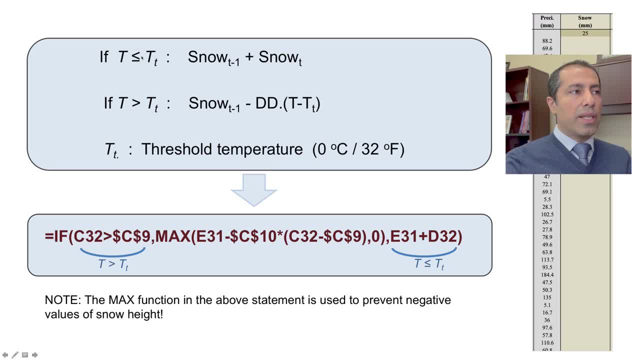 We need a two part equation like this: If temperature is below or equal temperature threshold, then simply snow at time T plus snow at the previous time, step T minus one. And if temperature is above snow from T minus one the previous time step minus snow melt. 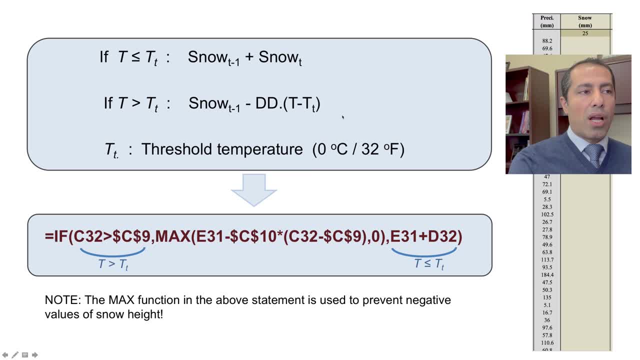 DD times. T minus temperature threshold describes snow melt and snow. T minus one is snow in the previous time step In day. one snow in the previous time step is our initial value. There is 25 millimeter of snow already on the ground. 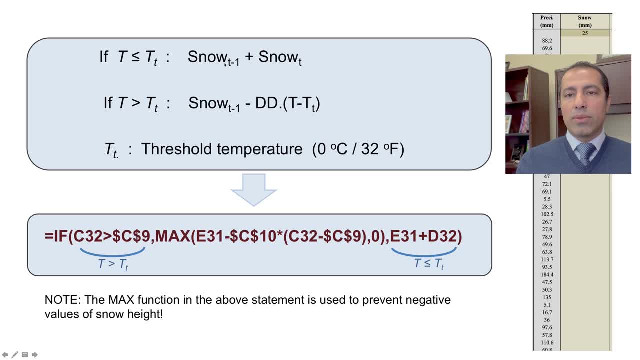 That's our T minus one. If there is no snow, there is no snow on the ground. Our initial value is zero for the first time step And we go forward day by day and we calculate snow accumulation. The first seven days temperature is below zero. 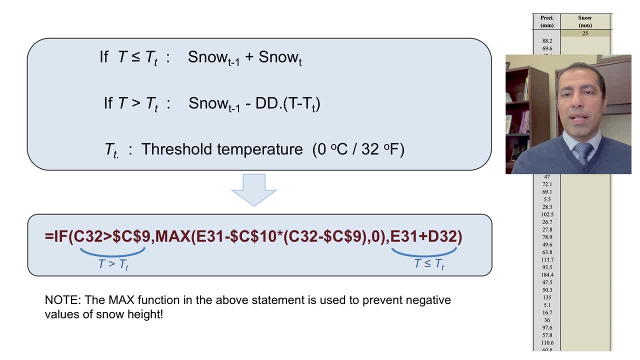 It means we just add snow values. So we calculate snow accumulation. There is no snow melt, but day eight in the model temperature exceeds the freezing level. It means we have rainfall plus snow melt. So we've switched to the second equation. We calculate snow from the previous time, step minus snow melt. 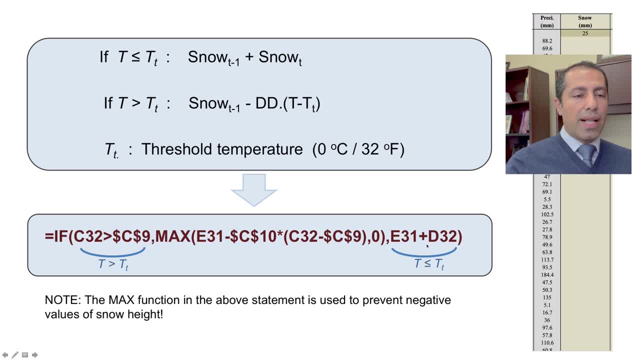 This is the equation that we need to use to calculate snow. We use an if function because we have a two part equation In an if function. you have a statement here. This is your main statement: temperature above temperature threshold. If this is true, 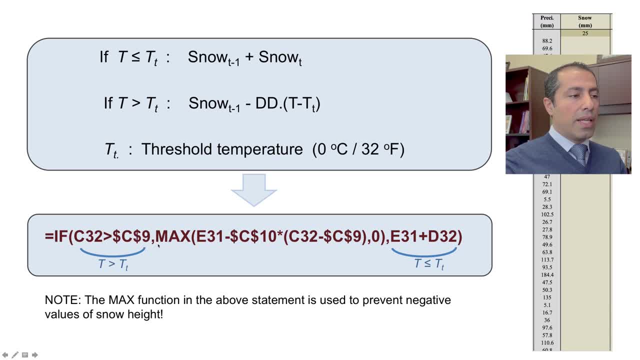 Excel will execute the first statement here. If false, it will execute the second. So if temperature is not above zero or temperature threshold, then we simply add snow values. So this part of the equation is the first part of our equation. So this part of the equation is the first part of our equation. 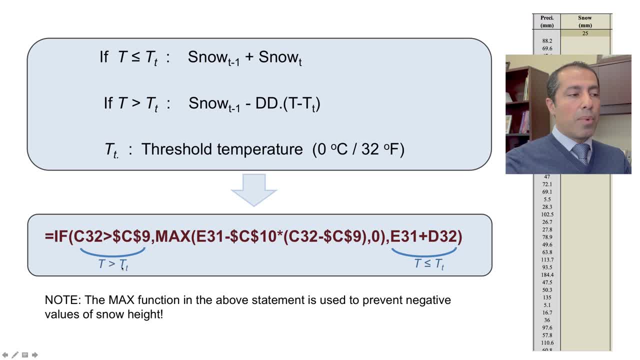 If temperature is above zero. If temperature is above zero, we have to calculate snow minus snow melt. But here we use a maximum function because we want to avoid negative values. Imagine there is five millimeter of snow on the ground And your degree day factor is 10 millimeters. 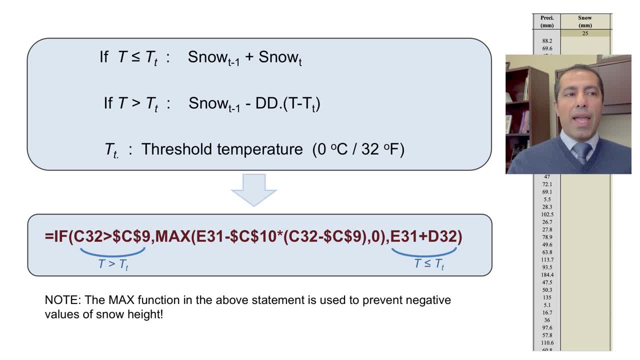 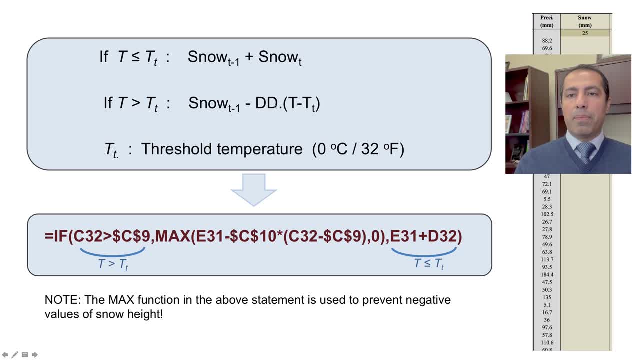 but 10 millimeter of snow melt per degree per day, Then the second statement will be minus five. but minus five snow doesn't make sense. If there is five millimeter snow on the ground, maximum amount of snow melt can be five millimeter. 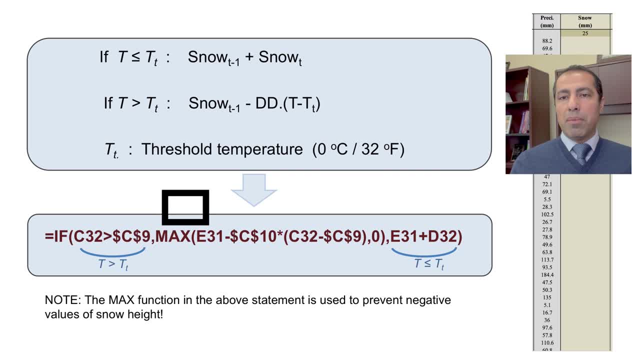 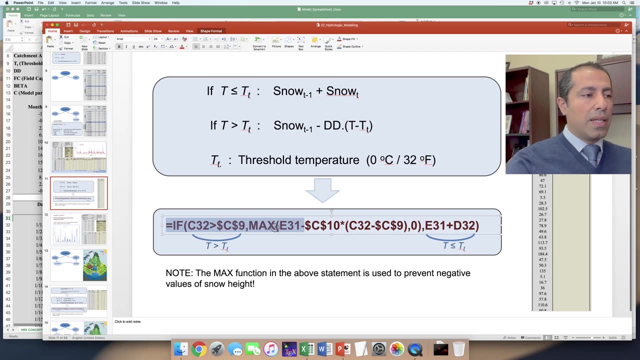 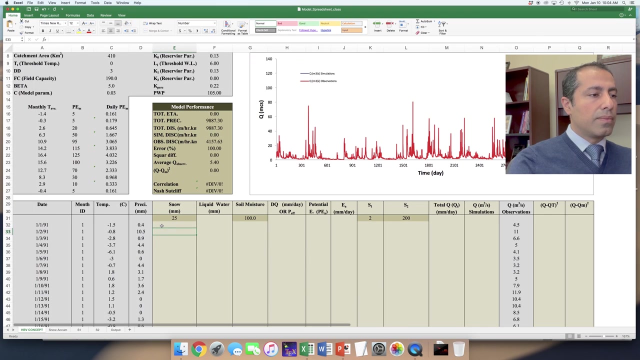 So degree-day factor is what can potentially melt, but if there is enough snow on the ground. So this maximum function here makes sure that we don't end up with negative snow values. Let's do that together. Let's apply the same equation to all rows. 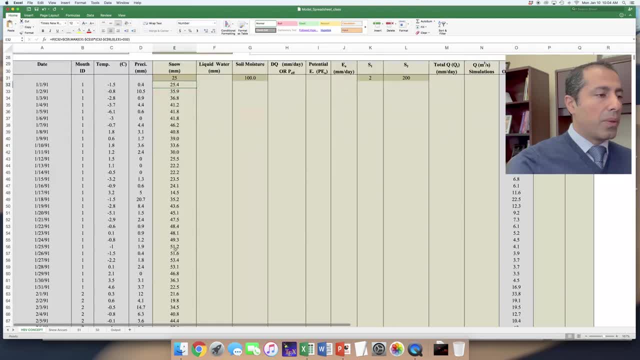 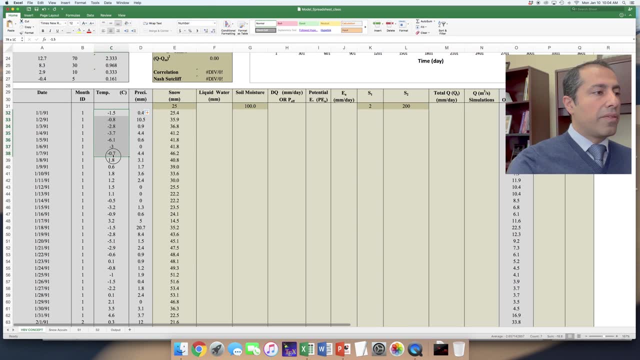 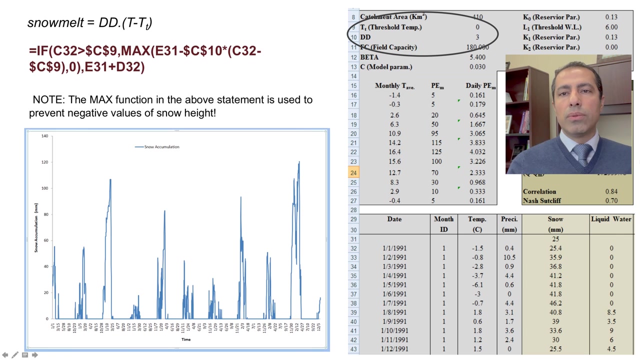 Now we have snow values throughout the entire period. As you can see, in the first seven days temperature is below zero and snow only accumulates. Then, when it goes above, snow decreases because we have snowmelt. So far we have used two parameters. 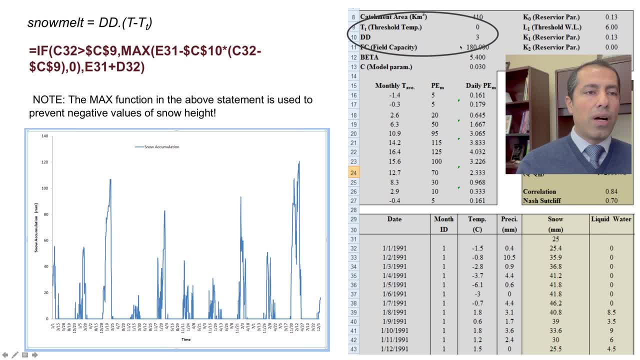 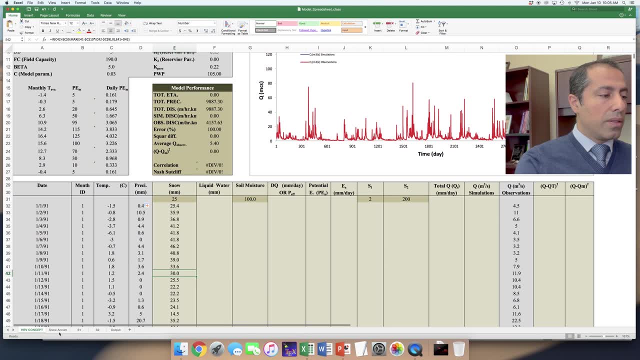 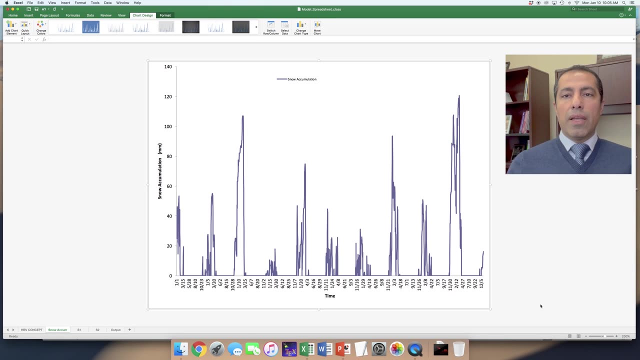 temperature threshold zero and degree day factor of three And we have calculated snow. We can always plot snow and investigate the time series and make sure it makes sense If you are in Northern hemisphere. in most parts of the world snow occurs in winter. 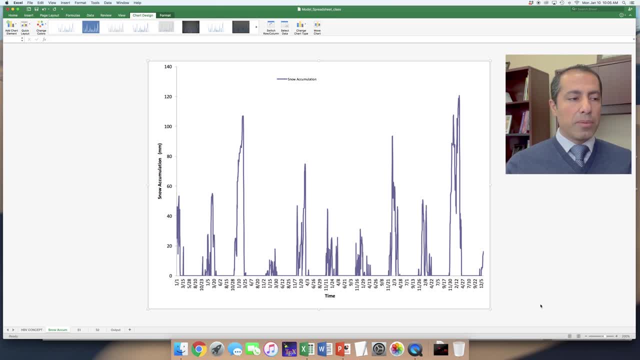 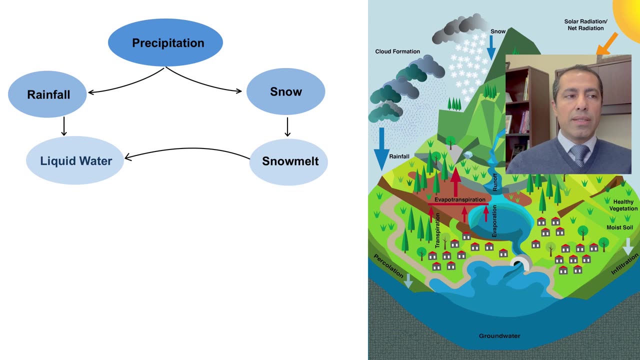 So you can look at your time series and make sure it's reasonable. This case snow looks reasonable. I have snow in winter and no snow in summer. We decomposed precipitation to rainfall and snow based on temperature and we calculated snowmelt. 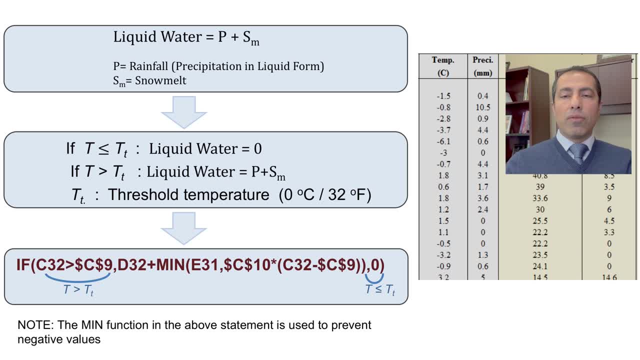 The next step is calculating liquid water. What is liquid water? Here we define liquid water as everything available in liquid form: Rainfall plus snowmelt. To calculate liquid water we have to make a simplifying assumption. Our assumption here is consistent. 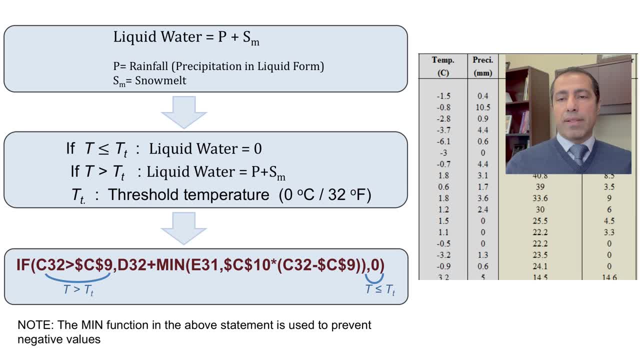 with the way we calculated snow and snowmelt. We assume if temperature is equal or below freezing level, liquid water is equal to zero. That means everything is frozen, And if temperature is above zero, then precipitation P. everything falls in form of rain. 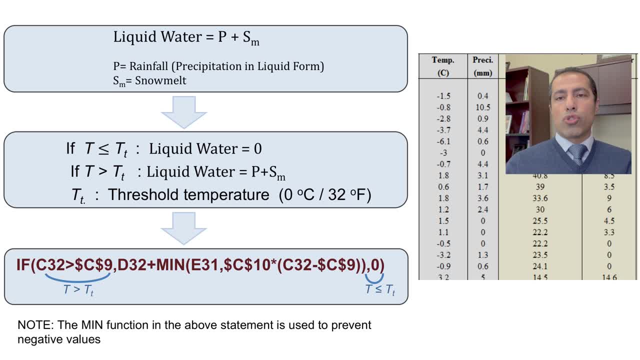 plus snowmelt SM. This is a very strong assumption, but when we don't have detailed data, we have to make simplifying assumptions. Also, this simple assumption allows us to minimize the number of parameters we need for hydrologic modeling. 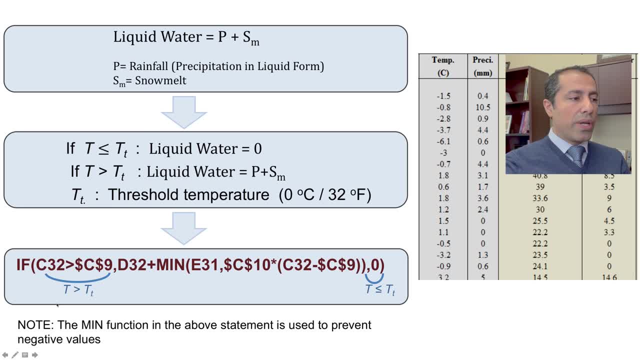 We use another if function, because we have a two-part equation. Our statement is: if T temperature is larger than temperature threshold, If true, the first statement will be executed. If true, the first statement will be executed. If false, then the second. 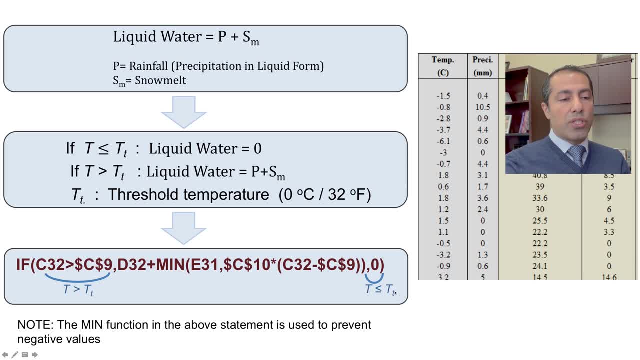 So the alternative, the second one, is T below temperature threshold. In that case there is no liquid water, So the statement is zero. And if T is above temperature threshold, D is precipitation. We assume it falls in form of rainfall plus snowmelt. 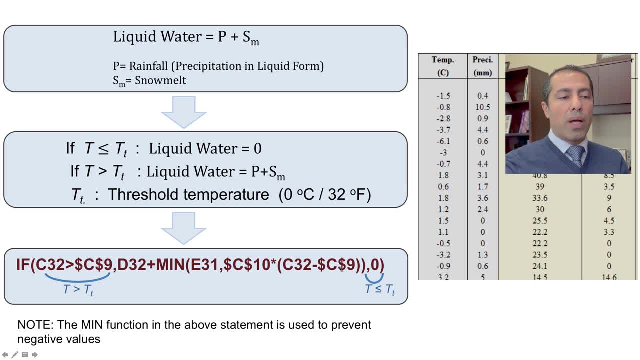 So snowmelt- here is degree-day factor times, the temperature. So snowmelt- here is degree-day factor times, the temperature. Similar to what I mentioned earlier. again, snowmelt depends on how much snow you have on the ground. Again, snowmelt depends on how much snow you have on the ground. 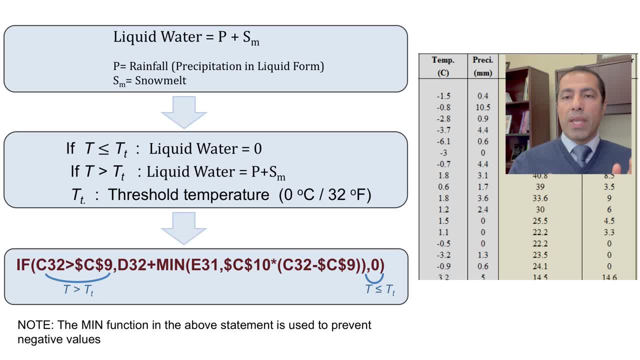 If there is no snow on the ground, there won't be any snowmelt. If there is five millimeter of snow on the ground and your snowmelt based on your degree-day factor is 10 millimeter, in practice only five millimeter of snow can happen. 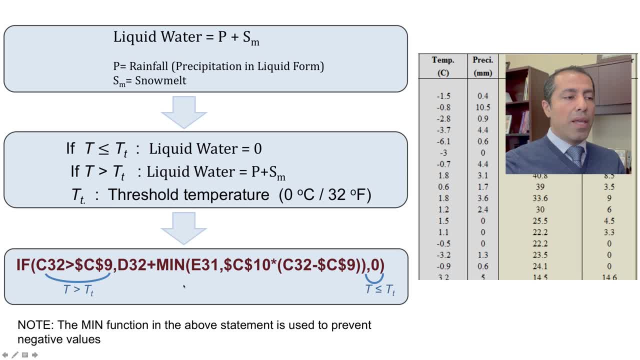 and no more than that. Because of that, because of the degree-day factor, we use a minimum function, because we want to avoid unrealistic snowmelt values. Also, note that in our equations we are fixing our parameters. Here, C9 is our temperature threshold. 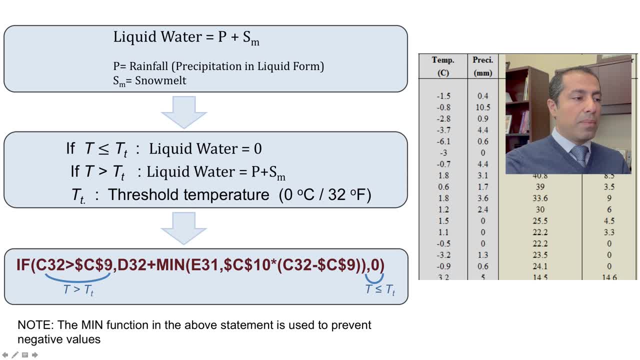 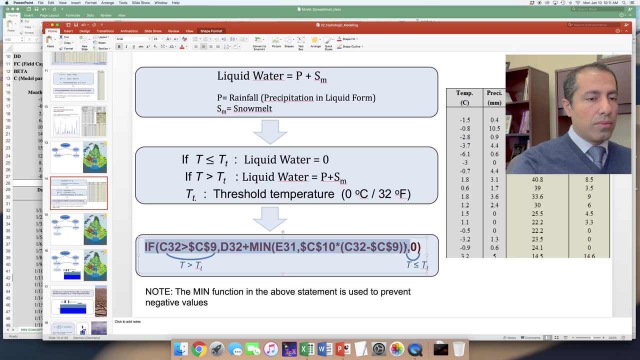 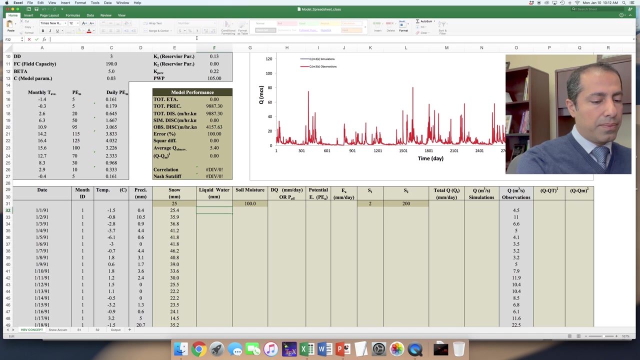 and the dollar signs means we have fixed them. It means, as we apply the same equation to other rows in our Excel spreadsheet, this value does not change, but temperature changes from day to day. Let's apply this equation In the first seven days. 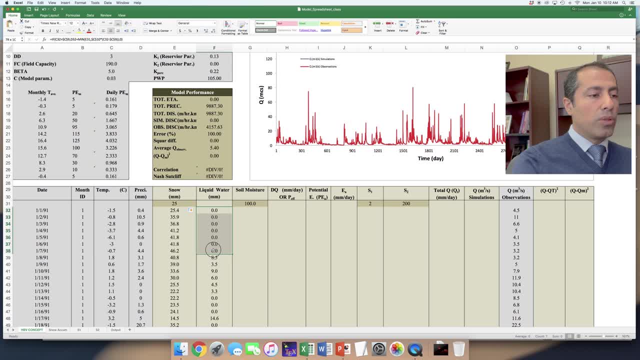 temperature values are below zero and there is no liquid water. And as soon as temperature increases and there is no liquid water, and as soon as temperature increases above the freezing threshold, then you see liquid water in your Excel spreadsheet. We used very simple models. 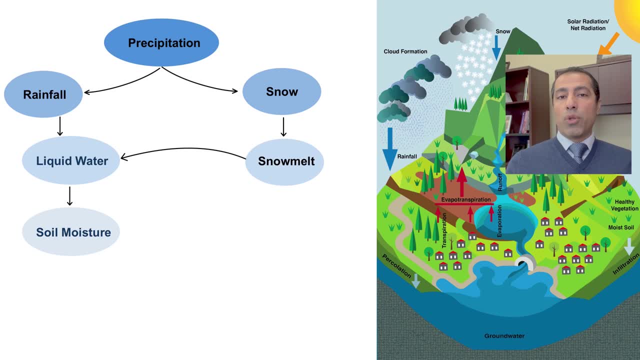 to calculate snowmelt and liquid water. Some snow models require more parameters, require more data, but here we are using one out of many models out there. There are other alternatives and you can change the model structure if you want. The next step is calculating soil moisture. 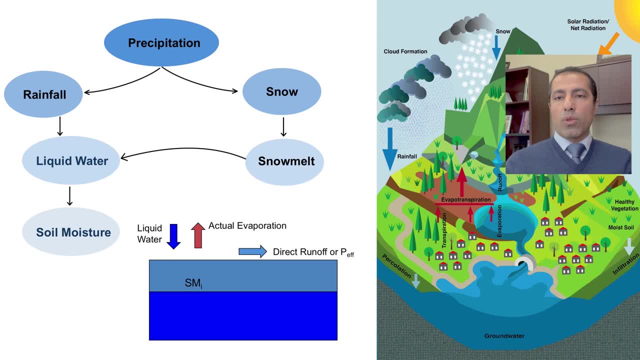 The next step is calculating soil moisture. For soil moisture similar to snowmelt, there are many different models out there. We use a simple water budget approach. Imagine the subsurface as a bucket Liquid water is like input into this system. 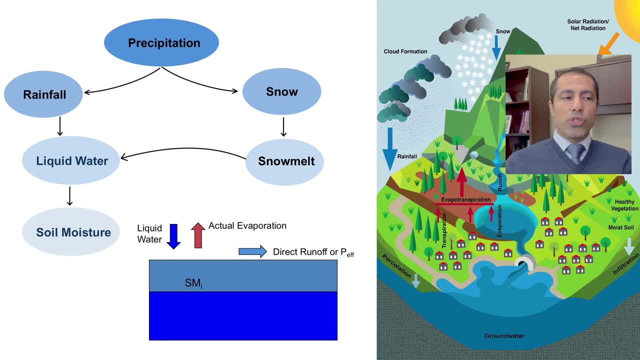 A fraction of liquid water contributes to soil moisture and a fraction of liquid water contributes to direct runoff. Here we also call it effective, Effective precipitation. In this presentation we use direct runoff and effective precipitation interchangeably, And actual evapotranspiration is a loss from the system. 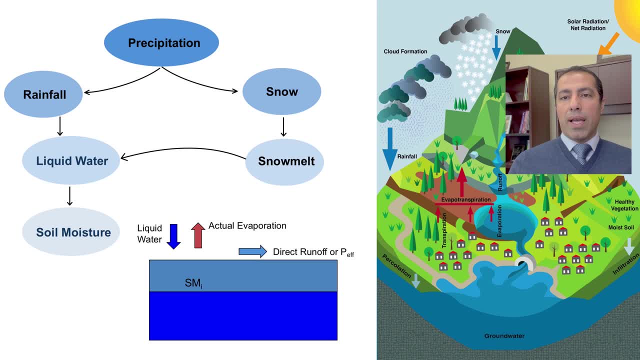 We know that water evaporates from soil and soil loses moisture through this process. You have input and output, So the main input is liquid water. The main outgoing flow is actual evapotranspiration. We also assume that there is. we assume that there is. 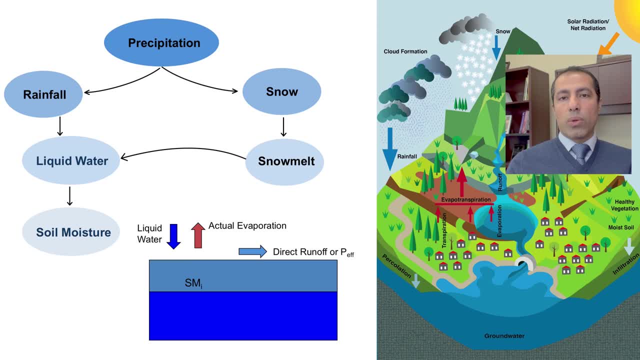 some amount of moisture already in the soil. Even during droughts and dry conditions, there is always some moisture in soil. So that would be our initial value, SMI, or initial value of soil moisture. That's the amount of moisture already in the soil. 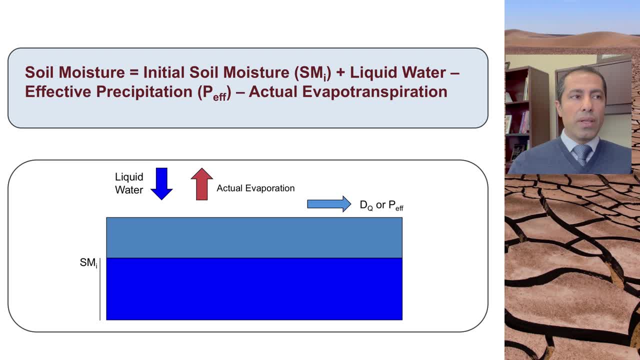 when you want to start modeling. So this is our general equation. It's very simple: Input plus initial value Input plus initial value. Input plus initial value Input is liquid water plus initial value of soil moisture minus effective precipitation. Why? 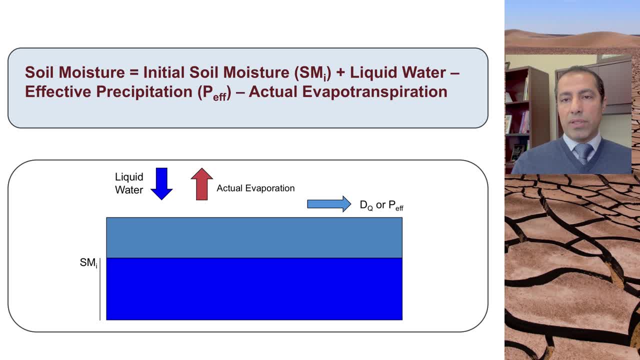 Because not all the liquid water infiltrates into subsurface. So liquid water minus effective precipitation is what contributes to soil moisture, minus actual evapotranspiration, which is loss in the system. So to calculate soil moisture using this model, we need to first calculate effective precipitation. 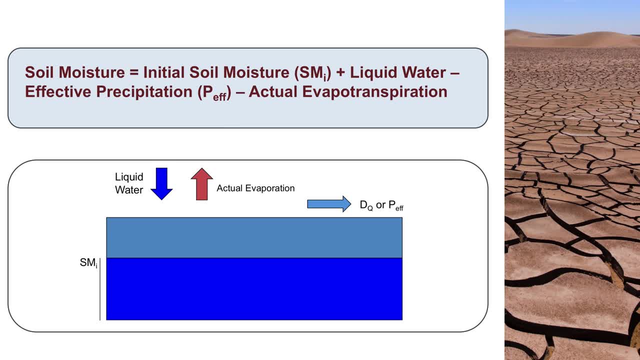 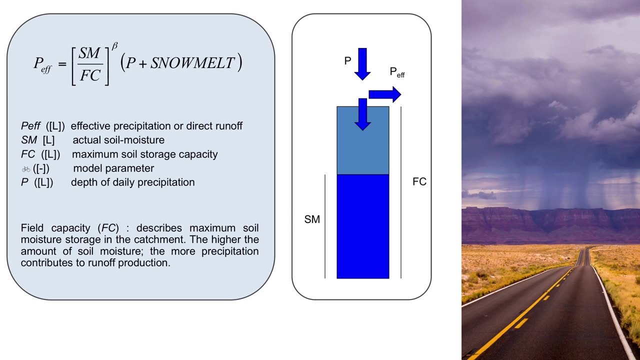 and then actual evapotranspiration. There are other soil moisture models that you can use, but this is our choice of model in this lecture. Let's start with effective precipitation. There are different methods. There are two methods out there to calculate effective precipitation. 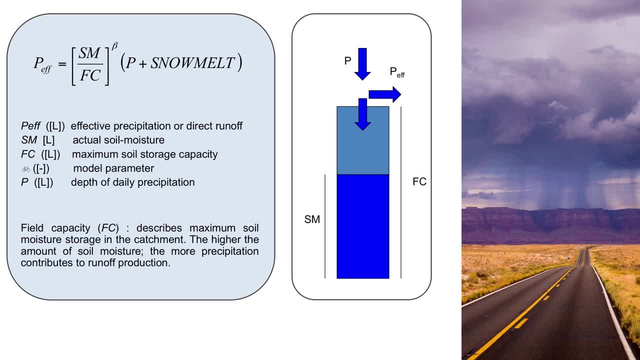 Here is one Soil moisture divided by field capacity: Fc to the power of beta times, precipitation plus snowmelt. Let's define these terms. Let's assume that subsurface is like a bucket- See the right figure here- And in this bucket, the capacity. 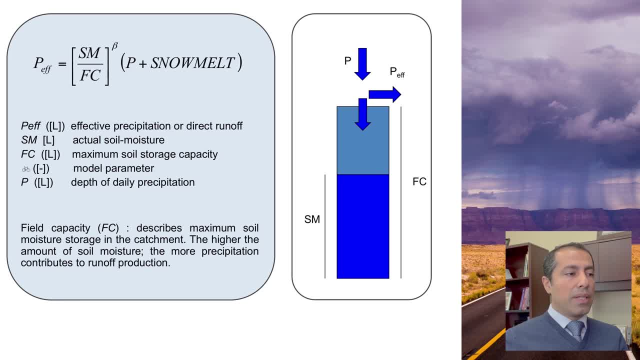 the maximum capacity is Fc or field capacity. Field capacity describes the maximum soil moisture storage in the watershed. So soil moisture can range from nothing to maximum of field capacity. So here field capacity is the upper bound for soil moisture. The higher the soil moisture, 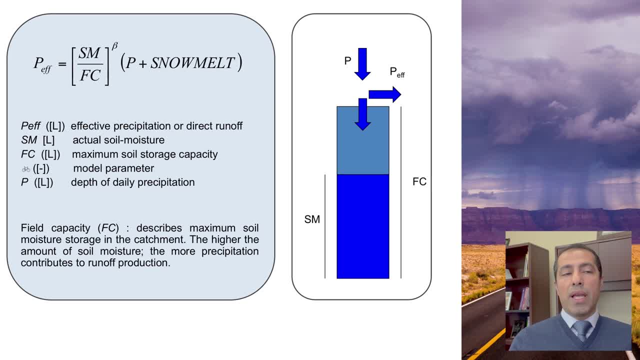 the less room is for infiltration and more water or more liquid water contributes to direct runoff or effective precipitation. If you look at this equation more carefully, P plus snowmelt is basically liquid water And of course, we only have effective precipitation in this model when there is liquid water. 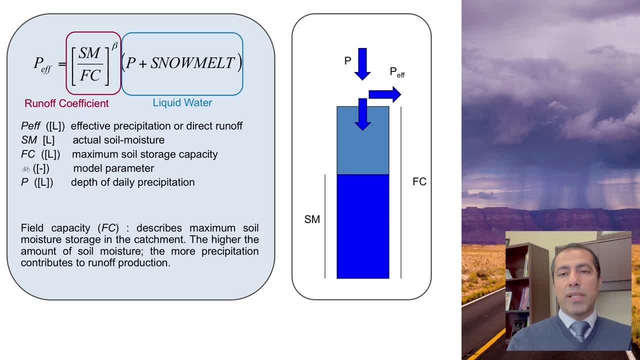 Remember, we made a simplifying assumption: If temperature is below zero, there is no liquid water And, of course, based on this equation, no effective precipitation. So the second part is liquid water And we have already calculated it. The first part, we can call it runoff coefficient. 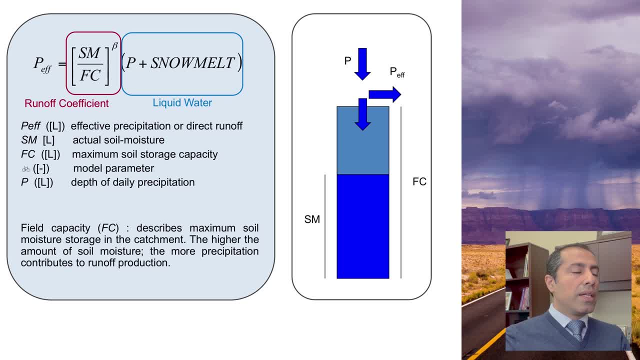 similar to runoff coefficient in other empirical method. Here the first term, soil moisture, divided by field capacity, ranges from 0 to 1.. When soil moisture is 0, runoff coefficient is 0.. When it is 1, it means soil moisture is at its upper bound. 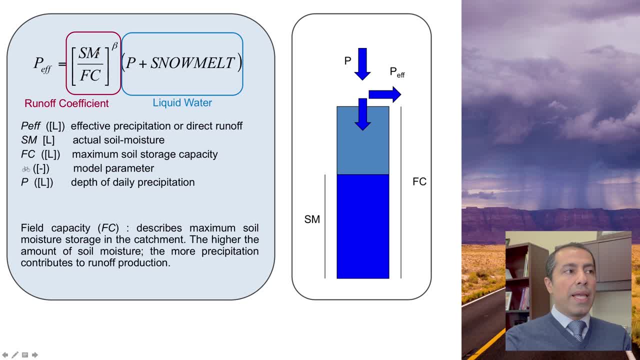 field capacity, So this term will be 1.. If this term is 1, it means there is no more room for infiltration or soil moisture is at the upper bound. Soil is fully saturated means the entire liquid water contributes to effective precipitation or direct runoff. 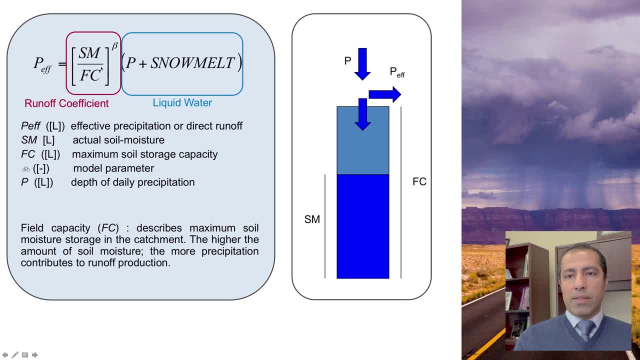 But if this term runoff coefficient is less than 0, then always a fraction of liquid water contributes to soil moisture. We can see the units here. For now all the variables are in unit length: Precipitation, snow, liquid water and also. 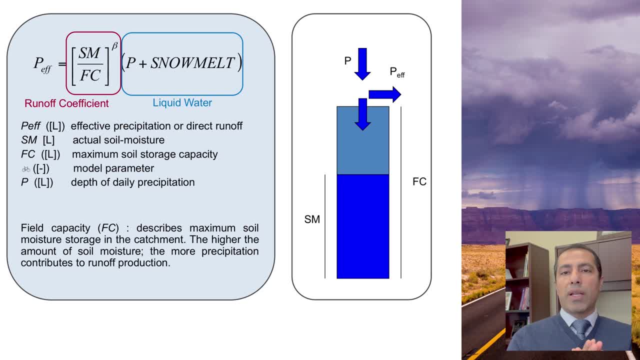 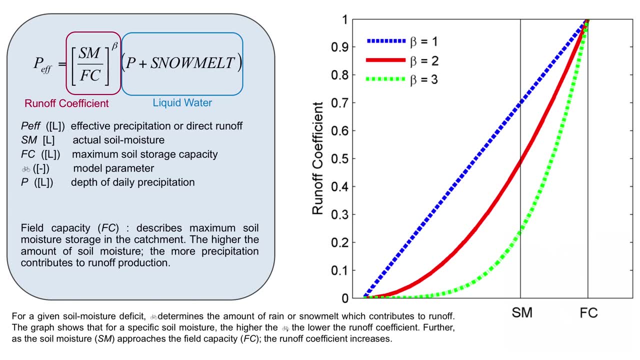 effective precipitation in our model are in unit length. We can always multiply by area of the watershed to calculate volume of water. If we plot runoff coefficient- the first term- against soil moisture in the x-axis, we can investigate the role of this parameter beta. 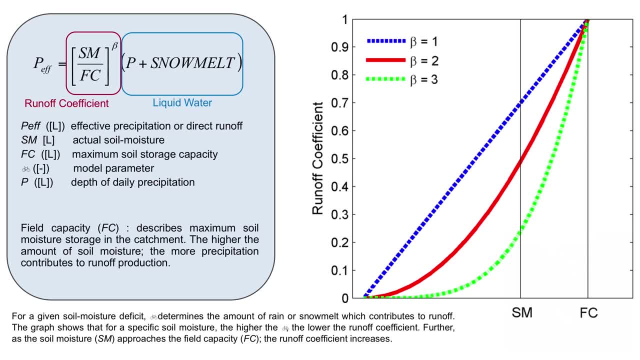 So the x-axis is soil moisture And remember it ranges from 0 to field capacity. Field capacity is like the upper bound for our soil moisture. Soil moisture also has unit length here, So this runoff coefficient is typically less than 1.. 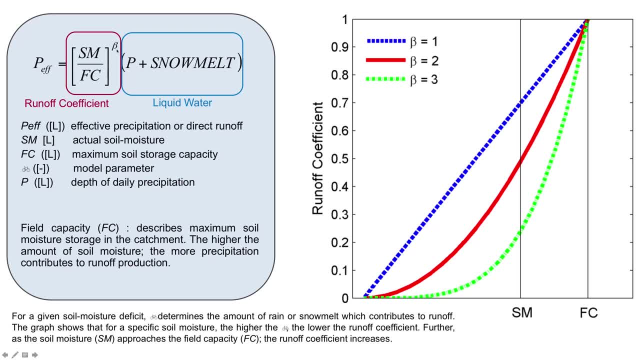 And if you raise a value less than 1 to the power of a value larger than 1, then it shrinks. So for beta equal to 1, we end up with a linear line like the blue dotted line here. 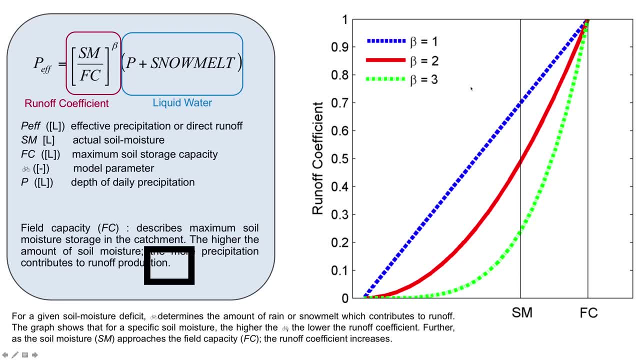 And if we increase beta to 2,, 3 or other variables, you see that this linear blue line turns into these red or green lines here and shows a non-linear behavior For a fixed amount of soil moisture. this vertical line movable. 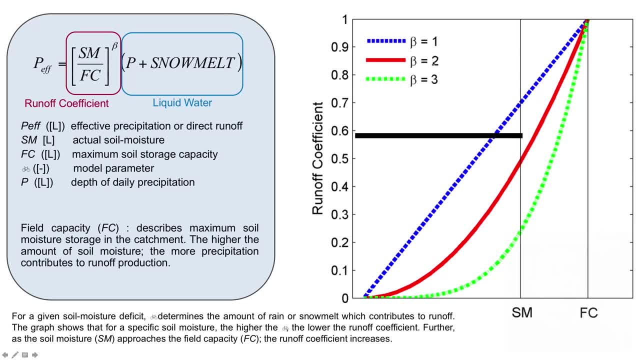 if we increase beta from one to two, runoff coefficient decreases. So if beta is equal to one, my runoff coefficient is 0.7.. If beta increases to two, runoff coefficient drops to 0.5.. And if it increases to three, runoff coefficient drops to 0.25.. Beta is simply. 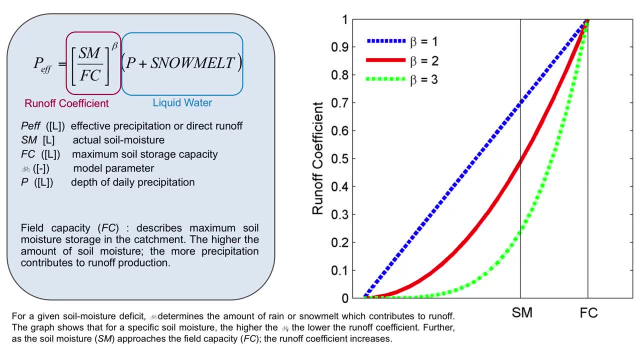 like a knob. It does not have a unit and it doesn't have any physical meaning here. It simply is a knob that allows us to change the amount of effective precipitation. Let's say, we start with beta equal to one and we notice that our model overestimates discharge One option. 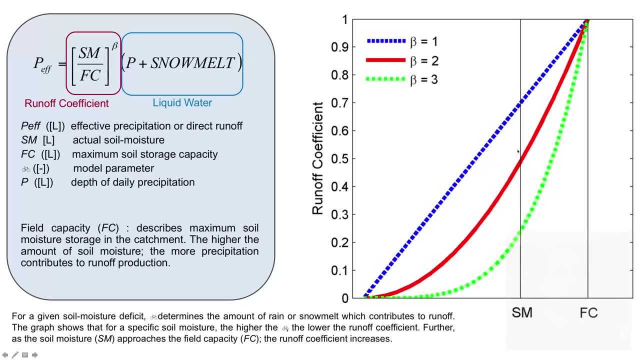 would be increasing beta so that we decrease runoff coefficient and runoff in our model. Later we will talk about this in more details, But here is an important point. The reason we are calculating effective precipitation is because we needed to calculate soil moisture. But we also need soil moisture to calculate effective precipitation. 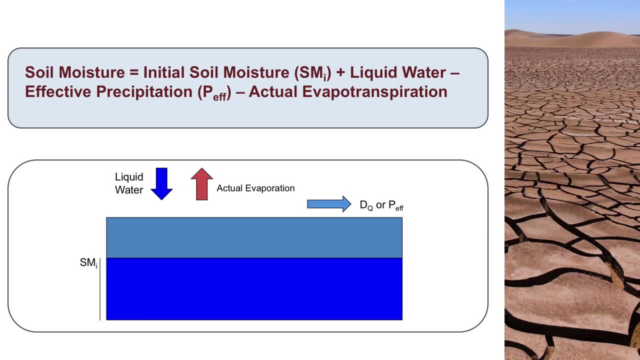 Let's look at our equation again. Soil moisture is equal to initial value of soil moisture plus liquid water, minus effective precipitation, minus actual evapotransmitters. But in our equation, to calculate effective precipitation, we need soil moisture too. Here again we have two variables that are linked together, in this case through soil moisture. 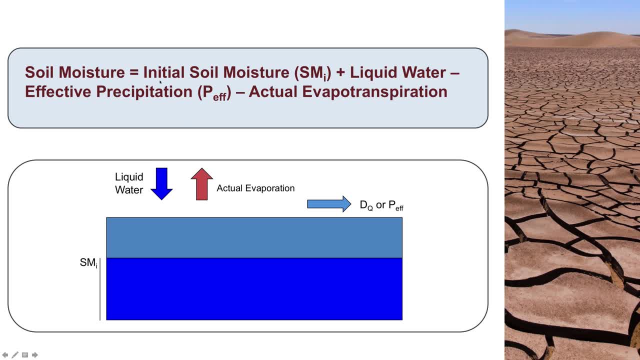 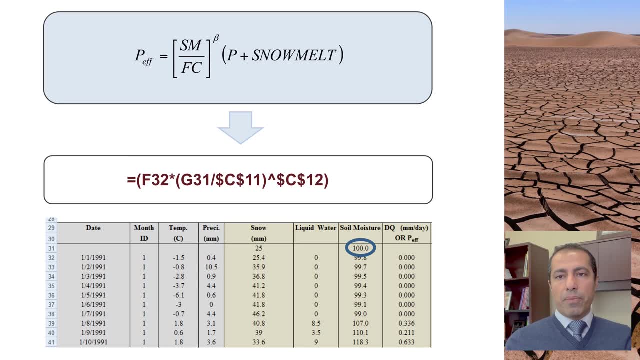 and we want to solve this problem. The way we approach this issue is using initial values or initial soil moisture. Again, we have to make an assumption. In our Excel spreadsheet there is an initial value for soil moisture. The value is 100.. Again, we are using unit. 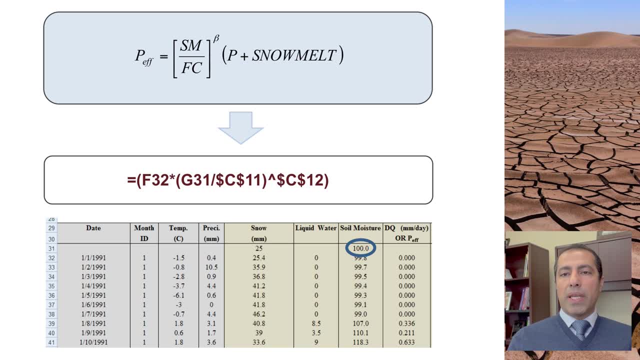 length for everything. So we are assuming that in our subsurface there is equivalent of 100 millimeter of soil moisture. Later we will revisit this assumption and we evaluate it. This is our equation. F32 is liquid water. that you have already calculated. 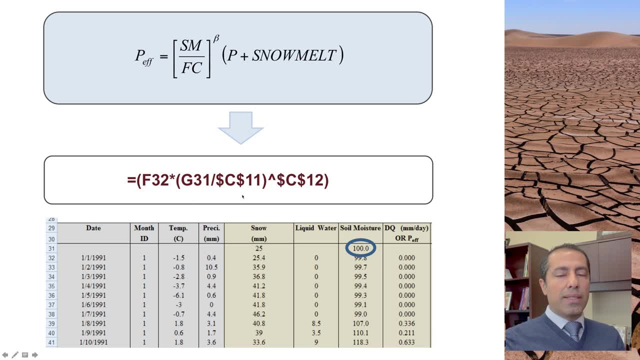 Soil moisture divided by field capacity. Field capacity, again, is a parameter. It's a physically based parameter that we can measure. But if you don't have any direct data, you need to make an assumption. For soil moisture we use the initial value, 100 divided by field. 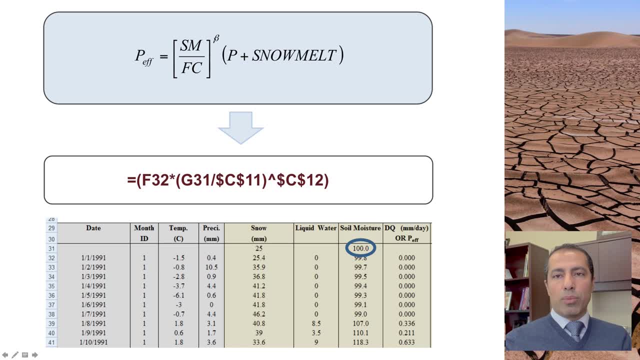 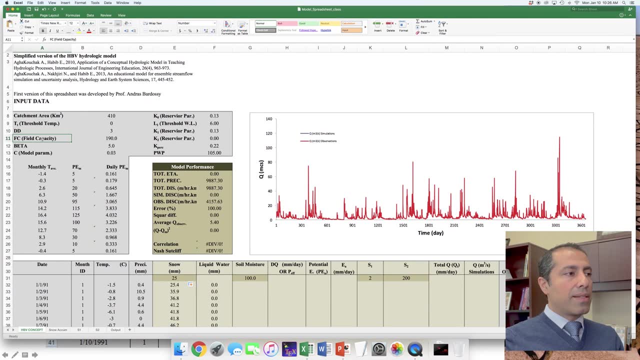 capacity to the power of beta. Again, for beta we have to make an assumption times: liquid water. Let's look at our Excel spreadsheet: Field capacity. our initial value is 190, and for beta we have used five. Effective precipitation is Kern edge. 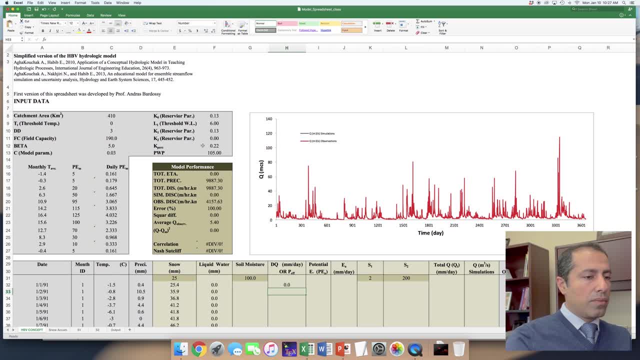 Our stock as H is true Overall, a gauge is minus Ypa And the data. we also already found that 3.. Kom2 is our banded Surface. The field capacity is zero. ents growth ratio is zero. Corral ripple coverage is zero. The last does not match Mcilla S sqrt value is zero. This is what you want to correct. Let's look at our Excel spreadsheet. Let's look at our Excel spreadsheet: field capacity: our initial value is 190 for beta. we have used five, So effective precipitation is con H. 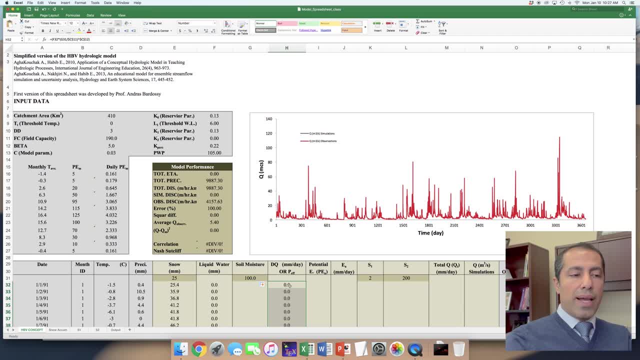 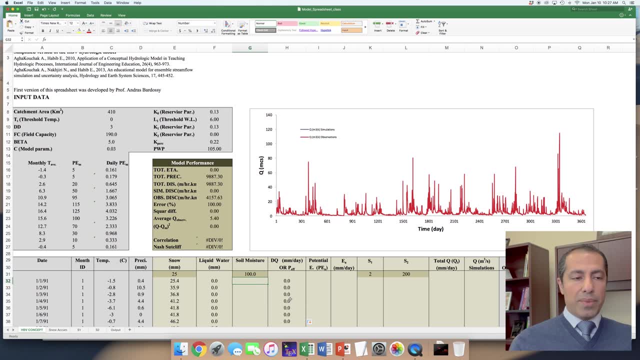 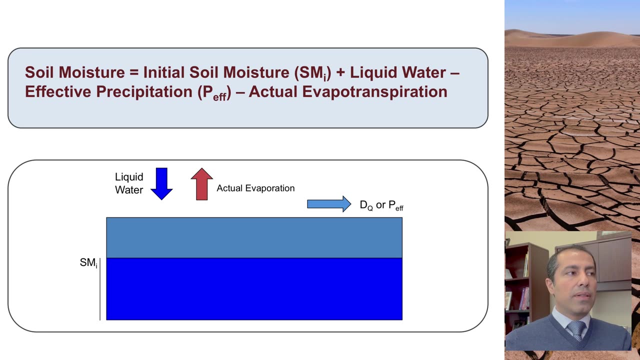 So effective precipitation is con H. Our values won't make sense right now because we don't have soil moisture yet. When we calculate soil moisture, all these values will be updated Back to our soil moisture equation. we calculated liquid water and effective precipitation. 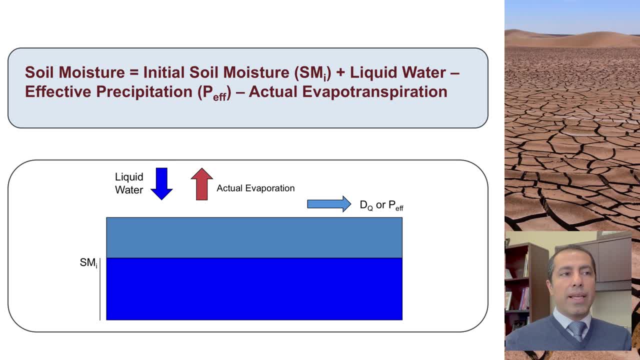 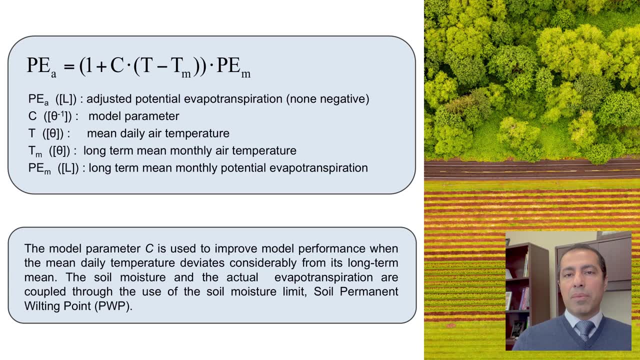 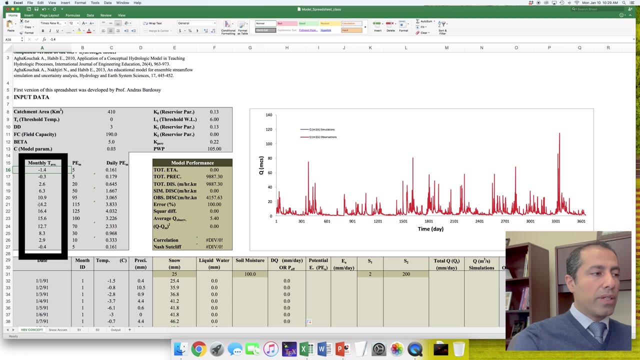 We assumed initial value of soil moisture. The next step is actual evapotranspiration. In our Excel spreadsheet we already have long-term average monthly potential evapotranspiration and also long-term average temperature. These 12 values here are average temperatures. 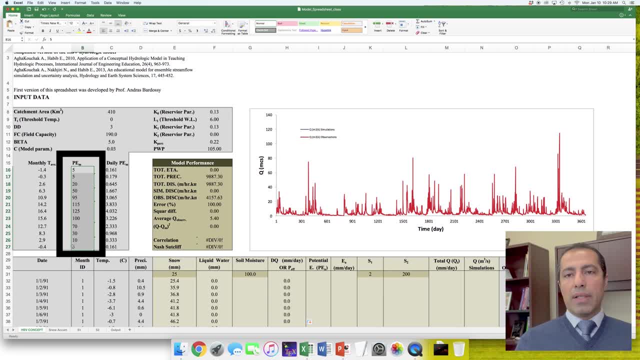 And these 12 values are average potential evapotranspiration at monthly scale. Potential evapotranspiration. Potential evapotranspiration is available from different data sets around the world, So if you don't have data, you can go to one of the existing data sets. 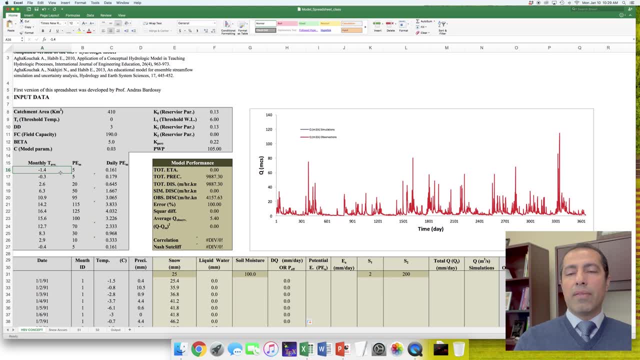 For example, NOAA, NASA and even some academic institutions have their own global potential evapotranspiration data. You can go extract data for your own basin. Long-term temperature, long-term monthly temperature are also available from multiple data sets. The third column here is daily equivalent of potential evapotranspiration. 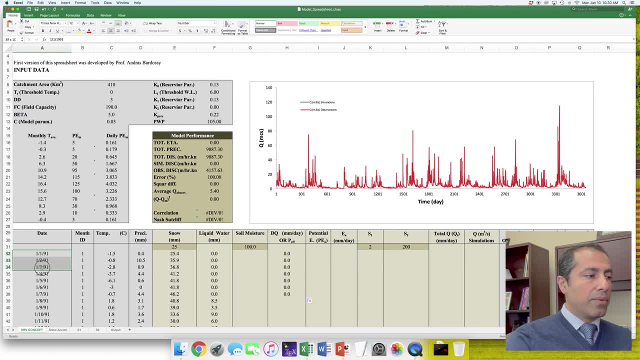 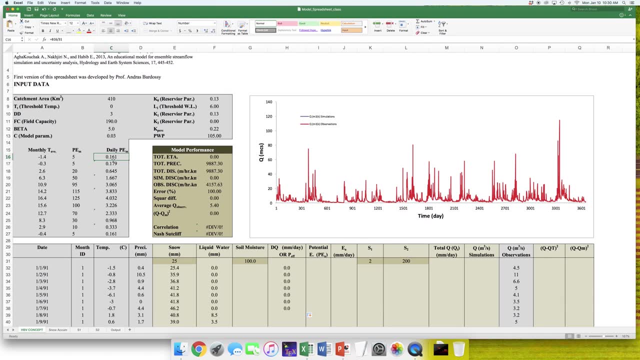 Here the temporal resolution of our model is daily. Every day we have temperature and precipitation, So for potential evapotranspiration we need to use daily equivalent. Basically, each value in the second column divided by number of days in that month gives you the equivalent daily. 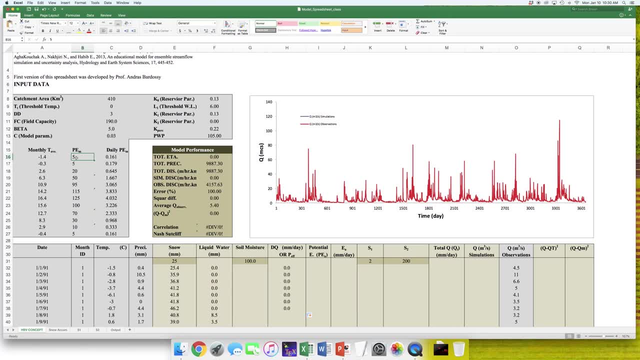 So 5 mm Per month in January means 5 divided by 31 days in January, you get the daily equivalent. The next value again: 5 divided by 28 days in February, you get the daily equivalent for all days in February. 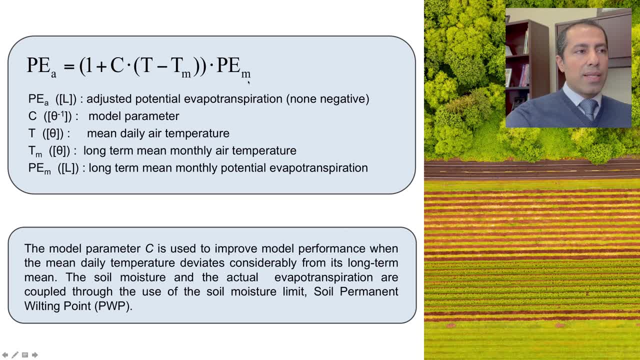 So in this equation potential evapotranspiration at monthly scale is available. It's an input variable Long-term temperature at monthly scale. Tm is also an input in our Excel spreadsheet And we want to adjust our potential evapotranspiration values for daily observations. 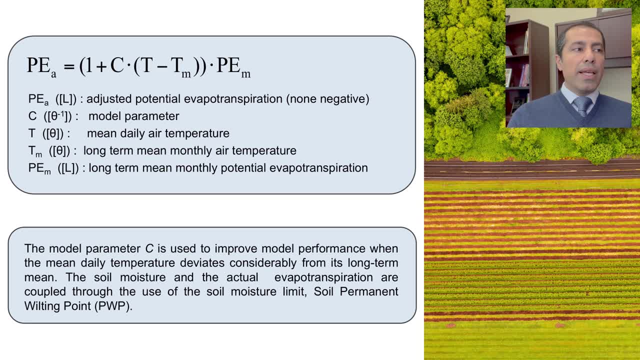 daily temperature observations in our study area. Again in this course. I assume you're familiar with fundamentals of hydrology and you know the difference between potential evapotranspiration and actual evapotranspiration. We don't go into details of PET or potential evapotranspiration. 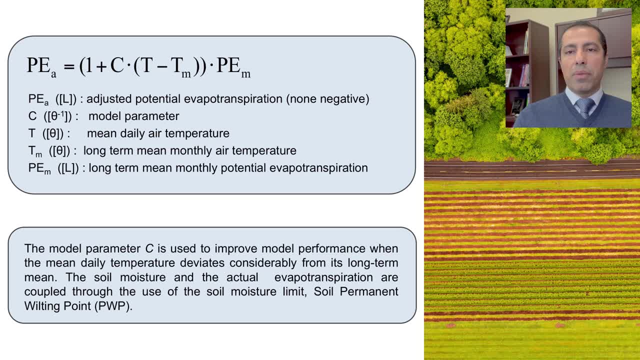 calculations. If you're not familiar with potential evapotranspiration estimation, I encourage you to review introductory hydrology textbooks to learn about different methods to calculate PET. Here we assume you already have potential evapotranspiration and you want to calculate actual evapotranspiration. 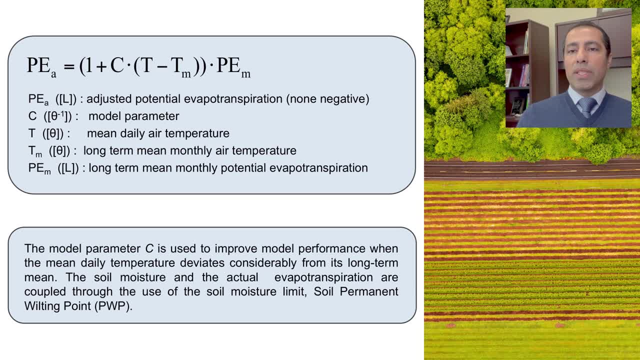 Very briefly, potential evapotranspiration is what can potentially evaporate it if there is enough water in the system, if there is enough water in the system, if there is enough water in the system and if there is enough energy for evapotranspiration. 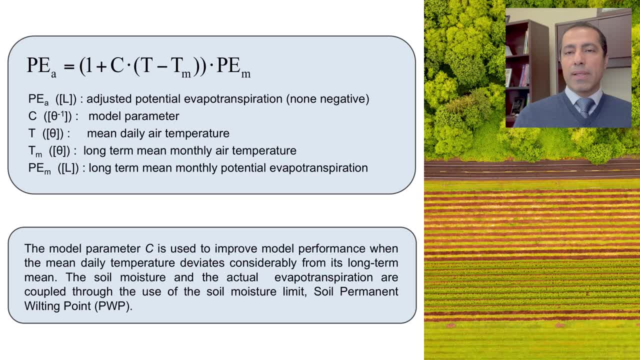 Actual evapotranspiration is what actually happens. So in theory, based on solar radiation, temperature and other variables in your study area, the potential evapotranspiration could be 100 mm per month. But if there is not 100 mm, let's say there is only equivalent of 20 mm of water. only 20 mm can get evaporated, So that would be 20 mm per month. So that would be 20 mm per month. There would be actual evapotranspiration and 100 would be the potential or the theoretical evapotranspiration. 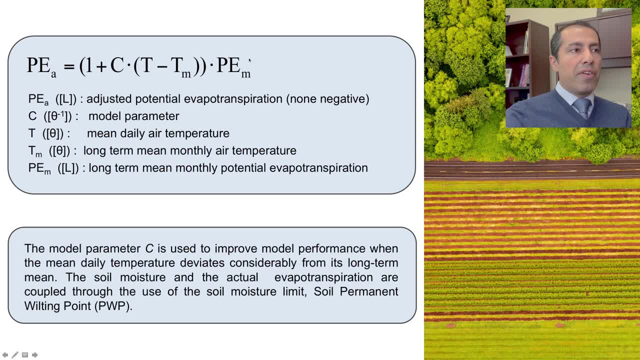 Here we have potential evapotranspiration. First we want to calculate adjusted potential evapotranspiration. That's PEA is adjusted potential evapotranspiration. What we calculate here is still theoretical. It is still potential, But we make adjustments based on daily temperatures. 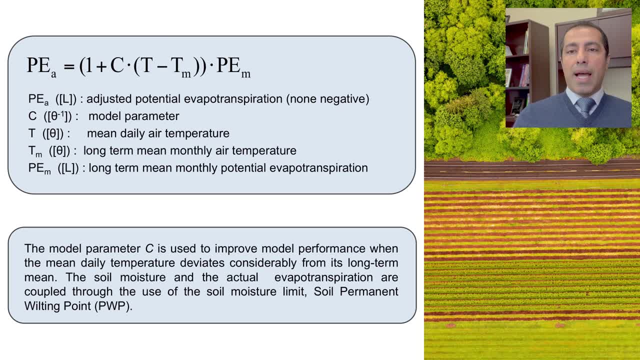 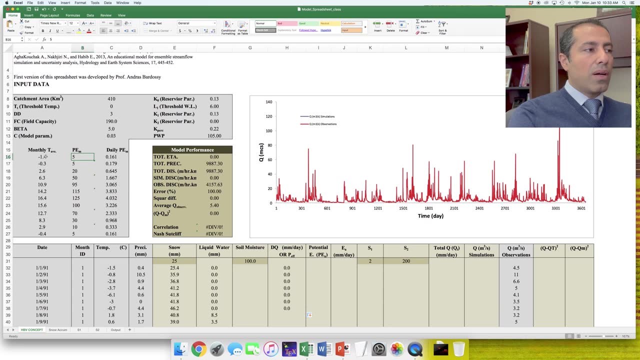 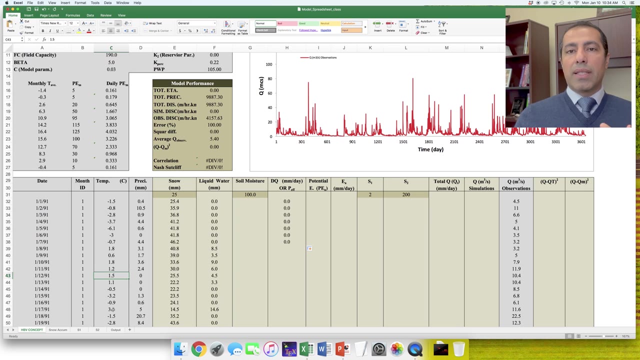 Our assumption is that our long-term potential evapotranspiration is primarily based on long-term temperatures. It means this value of potential evapotranspiration is based on long-term temperatures, So you want to make adjustments. If one day is much warmer than average temperature in January, you may want to adjust your potential and increase it. 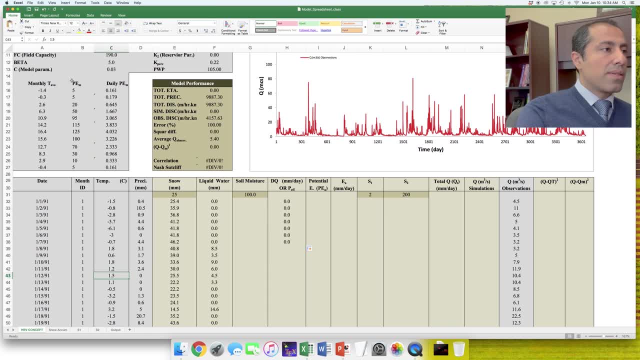 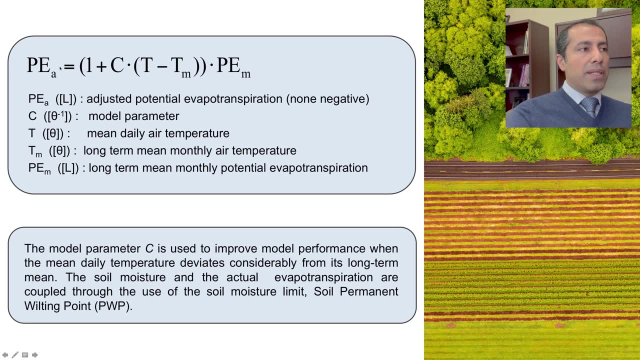 And if it is colder then you may want to adjust this long-term average and decrease it. So that's the point of adjustment here. So the adjustment is based on daily temperature difference: T, daily temperature minus long-term monthly. Long-term monthly temperature is the same for all values within each month. 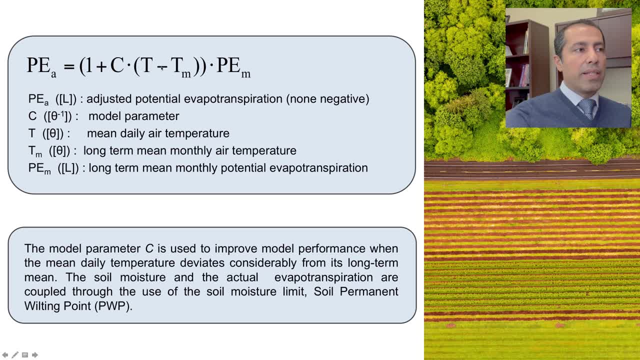 So all daily temperatures in January minus long-term January temperature Potential evapotranspiration at monthly scale is again the same for all values within each month. C is another model parameter. We have to make an assumption about C And then later we will do parameter analysis. 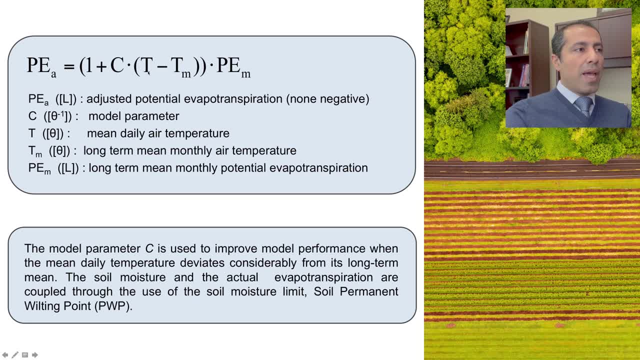 And then we will do our estimation and evaluate our assumption. So if temperature is larger than long-term temperature, this term will be positive. So adjusted potential evapotranspiration will be larger than potential evapotranspiration. If daily temperature is below long-term mean, this term will be smaller than one. 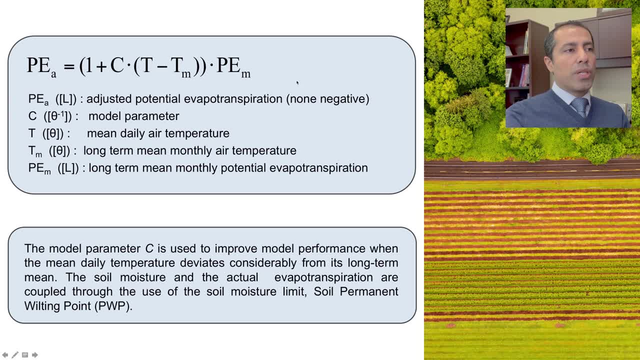 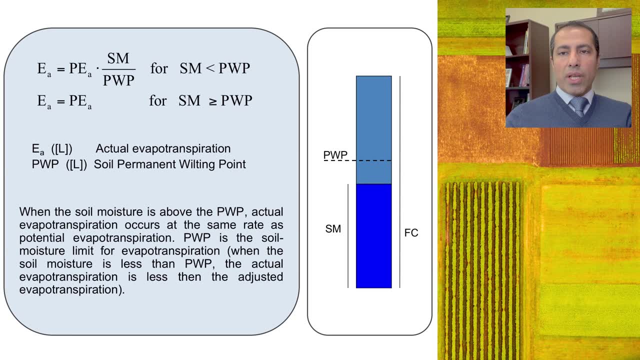 So adjusted potential evapotranspiration will be here. It will be less than long-term potential evapotranspiration. After calculating adjusted potential, we need to calculate actual evapotranspiration. For actual evapotranspiration we have to have a way to look into water availability. 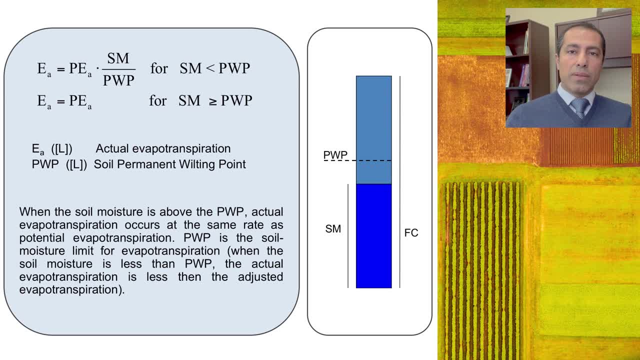 It means: is there enough water for evapotranspiration? If there is plenty of water for evapotranspiration, we assume that actual evapotranspiration is the same as potential evapotranspiration evapotranspiration. But if there is not enough water in the system, then we need a model to 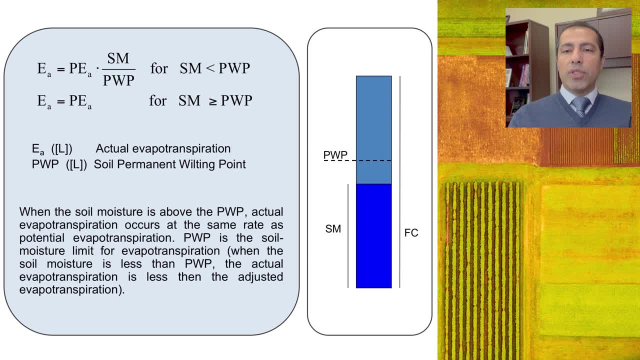 estimate actual evapotranspiration. Here we use another parameter for water availability. We call it PWP or permanent wilting point. Permanent wilting point is a threshold. We simply assume that if soil moisture is below permanent wilting point, then we are water limited. It means there. 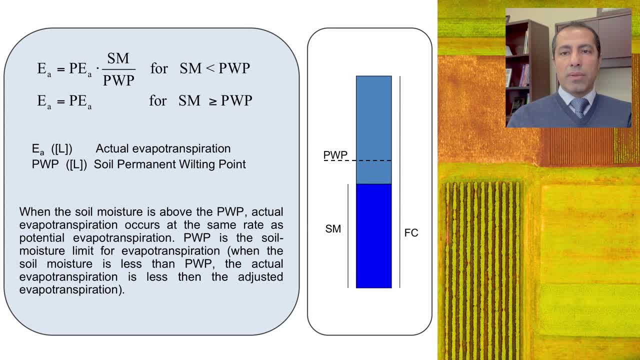 is not enough water for evapotranspiration to meet the potential. So actual evapotranspiration when soil moisture is below permanent wilting point is equal to adjusted potential, what you calculated in the previous time: step times: soil moisture divided by permanent wilting point. 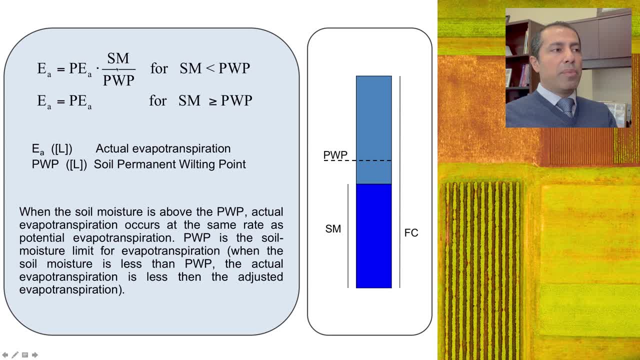 We use only this equation when soil moisture is below permanent wilting point. So this term, the second term, is a threshold. So if soil moisture is below permanent wilting point, the second term in the equation will be less than 1.. In that case actual evapotranspiration will be 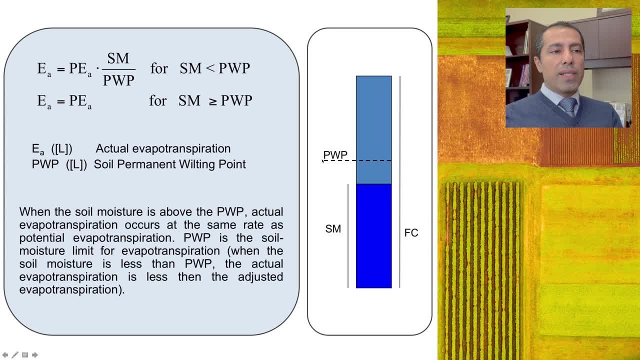 less than adjusted potential. But if soil moisture is above permanent wilting point, we assume there is plenty of water in the system and actual evapotranspiration is the same as adjusted potential. Again, this is a strong simplifying assumption, but it allows us to. 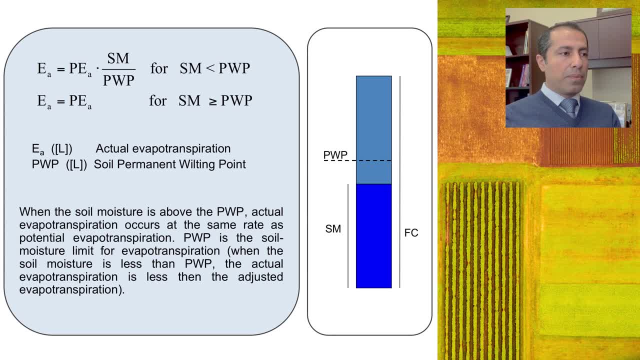 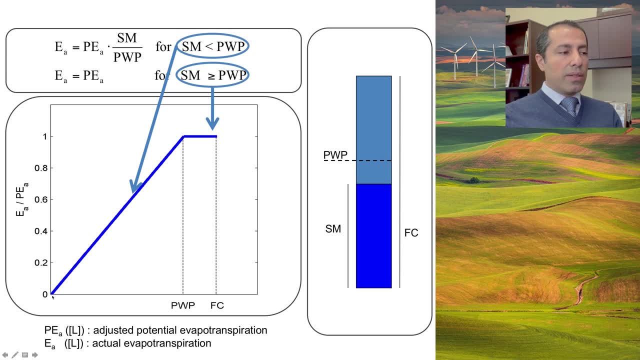 these variables with very few parameters. Here I am showing the equation graphically. The x-axis is soil moisture. Remember it ranges from zero to field capacity. Field capacity is the upper bound for soil moisture, so permanent wilting point PWP should be less than field capacity If soil moisture is above. 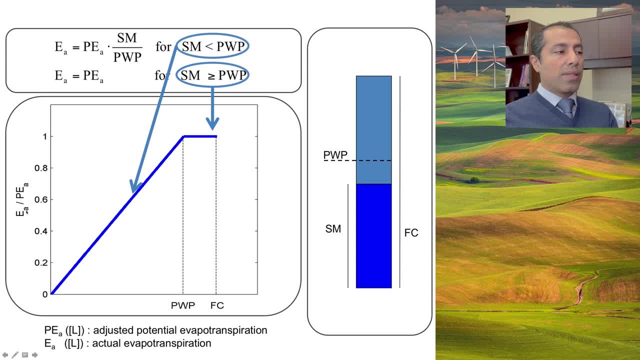 permanent wilting point. here in the y-axis we are showing actual evapotranspiration divided by adjusted potential. So in the first equation, if soil moisture is above permanent wilting point, then actual evapotranspiration is the same as adjusted potential evapotranspiration. So the ratio will be one straight line. 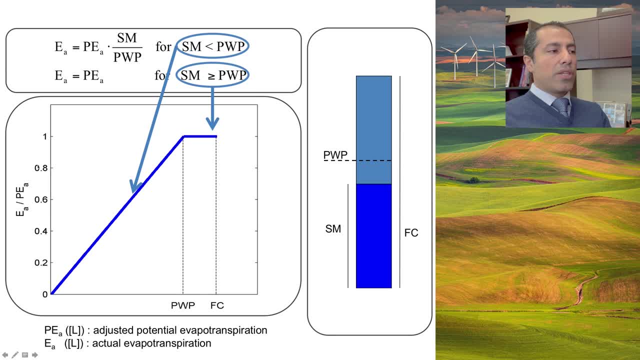 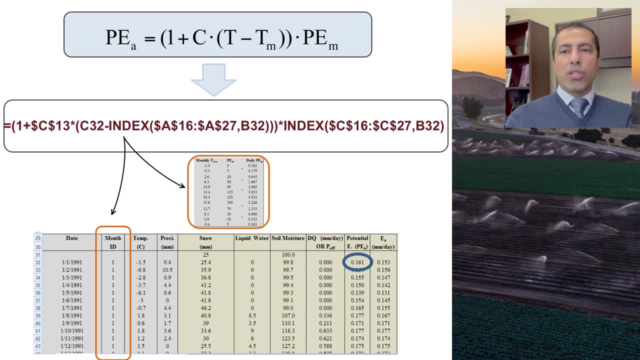 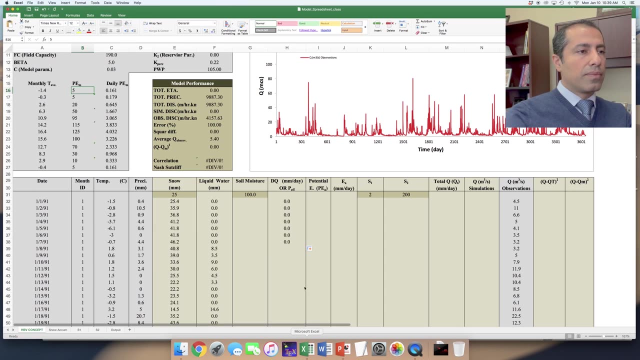 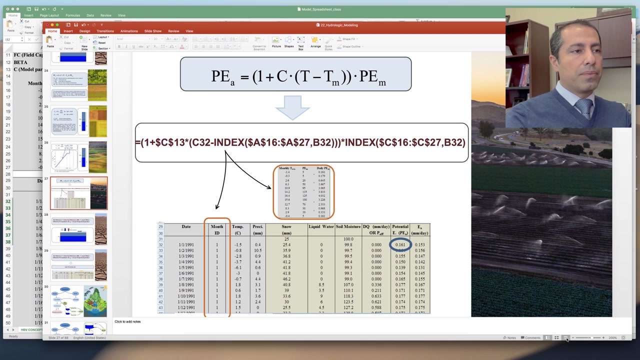 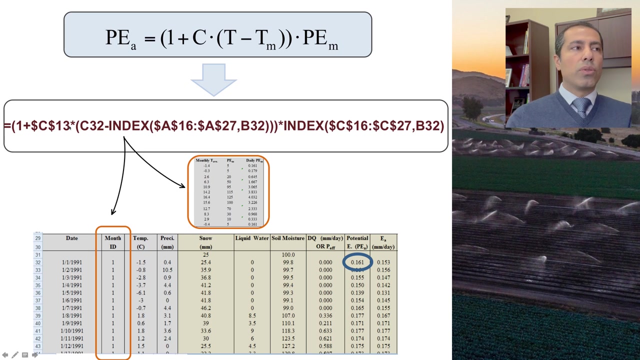 and if soil moisture is below this ratio changes linearly in this equation. Let's calculate adjusted potential evapotranspiration in our Excel spreadsheet. 1 plus C. 13 is our new parameter. It's a parameter. we need to calculate adjusted potential Parameter C. 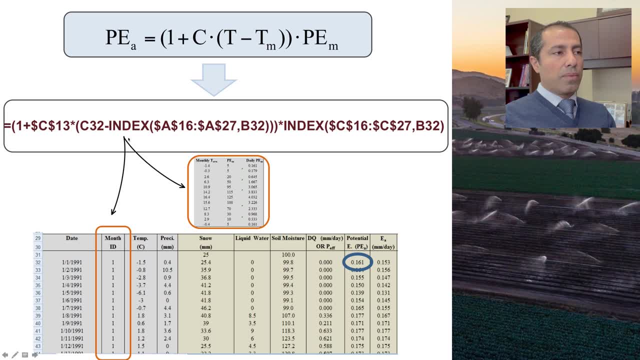 The method we are using here to calculate adjusted potential evapotranspiration has three functions: The first and the second. israhth function: the number of values minus the output variable and the figure of the value. This month you are doing an index function. Wanna start with the perfect equation. 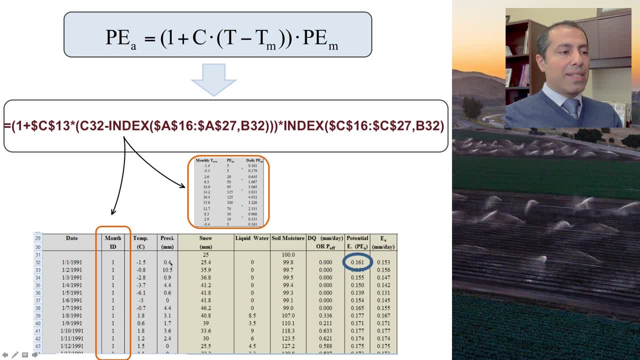 Review the syntax and learn how this function works. Here we have 12 values of monthly temperatures and also and also monthly potential evapotranspiration. Remember, for all January month we have the same average, January minus 1.4,. then the second day, again minus the same value and third day, again minus the same. 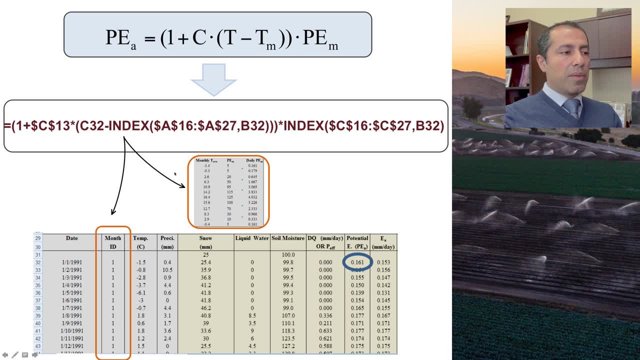 value Index function allows us to do that very simply and efficiently. So first we calculate month ID. So month function in Excel gives you the month ID, month ID 1,, 2,, 3.. So all Januaries in all 10 years we'll get the same month ID of 1.. All February month get month ID of 2.. Then the index. 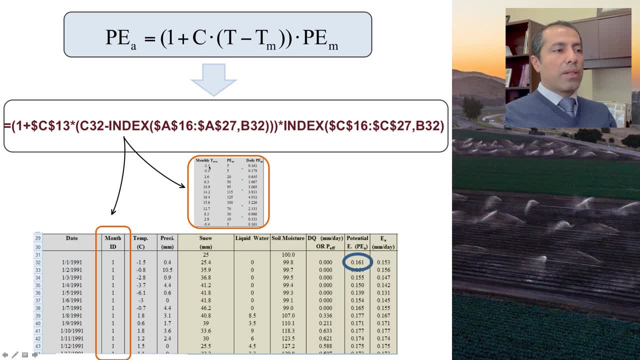 function tells Excel spreadsheet to subtract the right monthly temperature as you go through your time series. The same applies to potential evapotranspiration. Here we use the daily equivalent. Remember monthly potential divided by the number of days in that particular month, because our time step is daily. 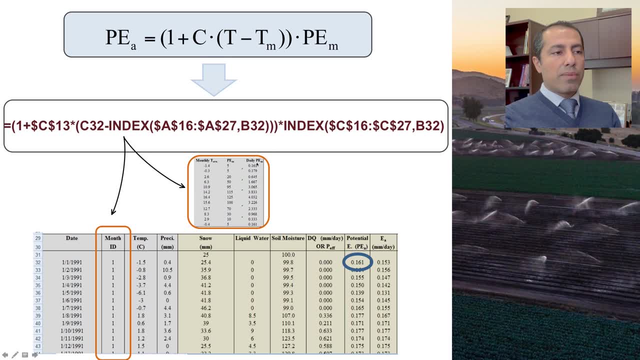 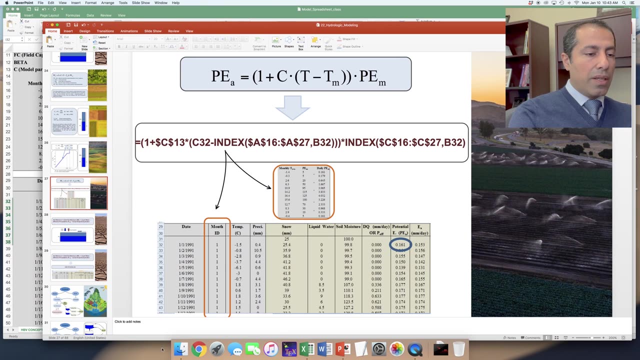 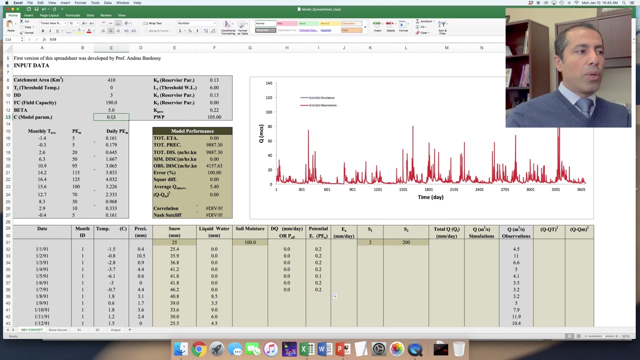 We select our 12 potential evapotranspiration values and the index is based on month ID. Here are our potential evapotranspiration values and the index is based on column B or month ID. If we look at our Excel spreadsheet, we are using this new parameter C 0.03, and these are our daily 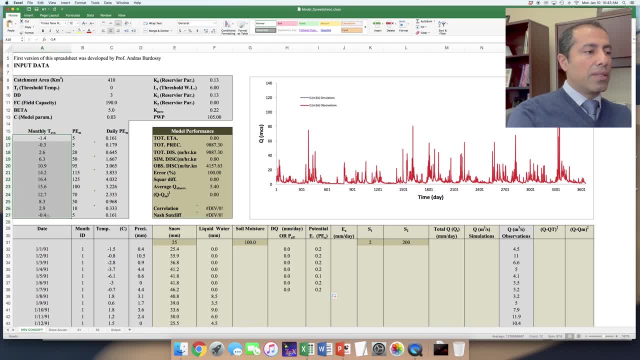 potential evapotranspiration values And monthly temperature values. The month ID is simply calculated using month function in Excel And if you click on the equation, you can see that you're using these monthly values of temperatures and potential evapotranspiration and month ID. If you go to day 2, now you're using 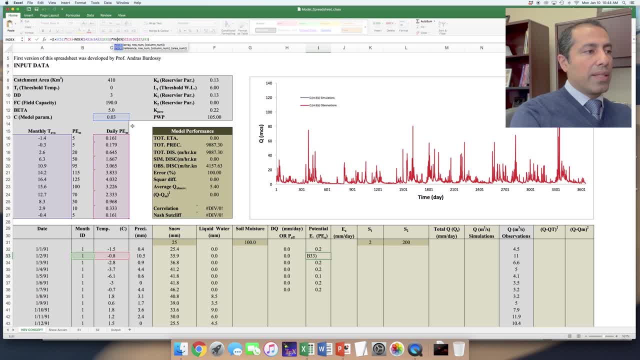 second day temperature. but these values remain the same And Excel knows that as long as the month ID is 1. It has to use the first temperature value here and the first evapotranspiration. When you go to month 2, it goes to the second temperature value and second evapotranspiration. 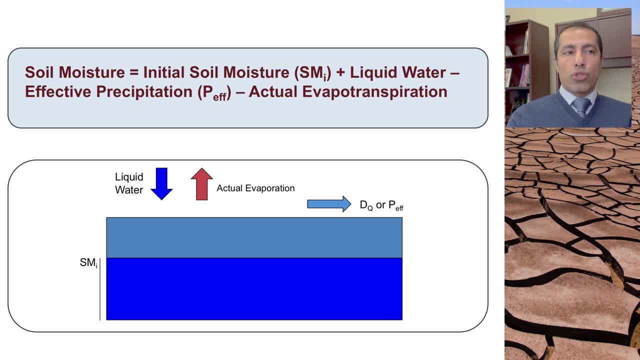 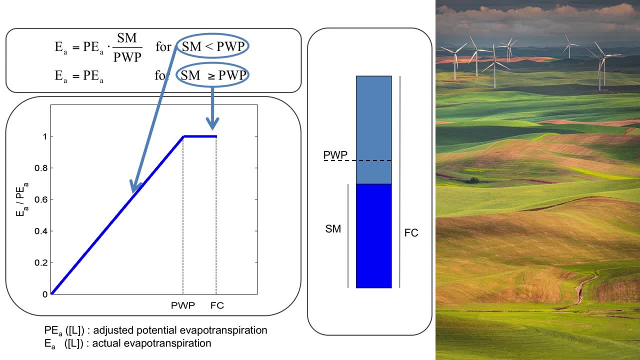 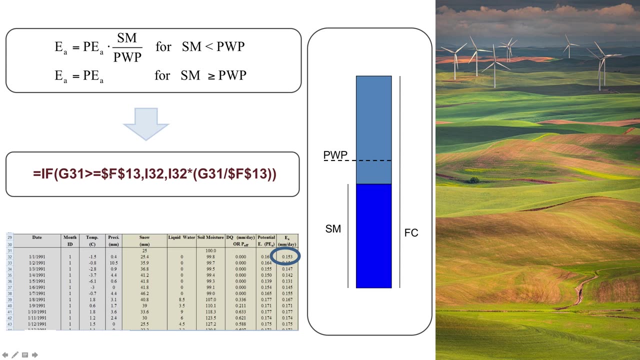 In our soil moisture equation. we need actual evapotranspiration and not adjusted potential. We need to update adjusted potential based on soil moisture and PWP. Here is the equation Again, another IF function: If soil moisture G31, is larger or equal to PWP F13,, then the first statement- actual evapotranspiration- is the same as adjusted potential. 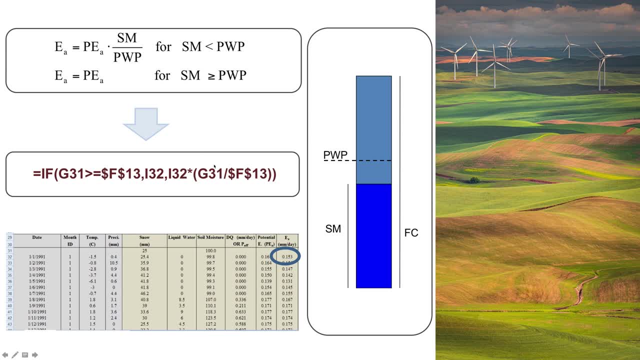 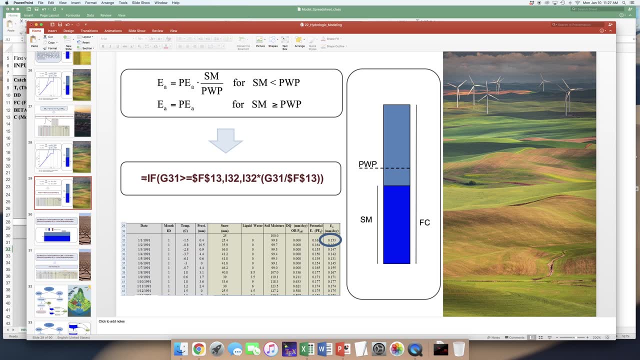 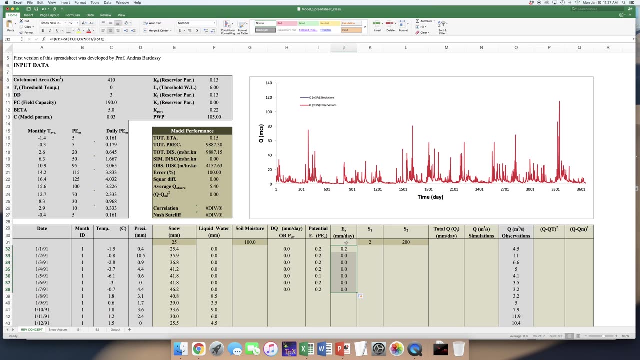 what we calculated in the previous time step. If not, we will calculate actual evapotranspiration using this equation here. Let's do this now. We need to follow step by step. Our values don't make sense yet because we don't have soil moisture. 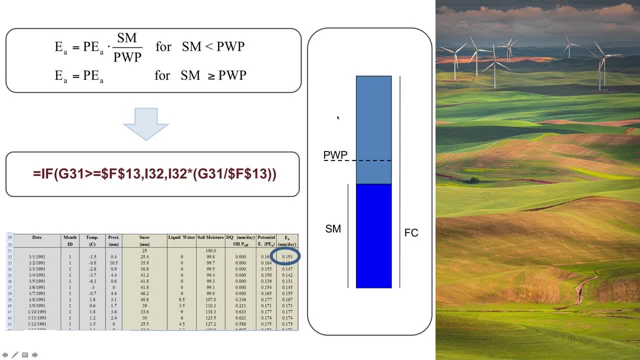 Remember, we are calculating actual evapotranspiration for soil moisture estimation. But, like in the previous step, we need soil moisture to calculate actual evapotranspiration. For the first time step, we use initial value of soil moisture. For the first time step, we use initial value of soil moisture. 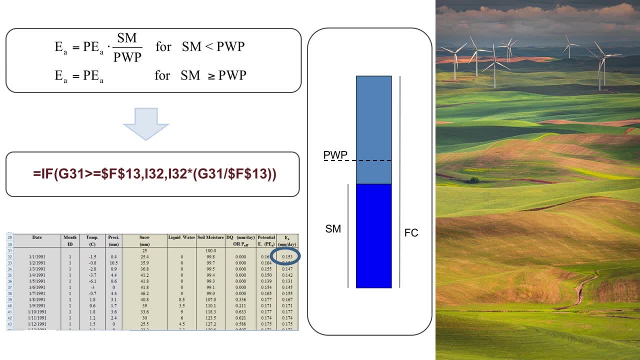 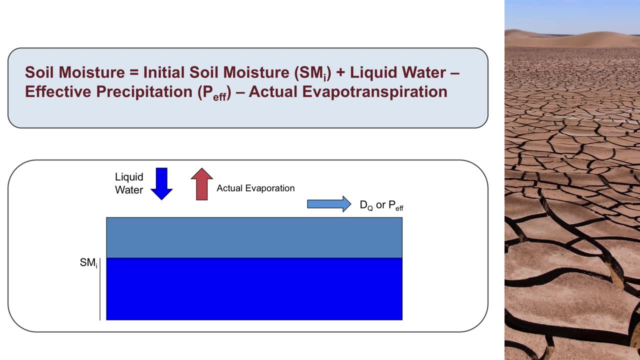 For the first time step, we use initial value of soil moisture. For the second day and more we don't have soil moisture yet, so our values for now don't make any sense, But they get updated Back to our soil moisture equation. 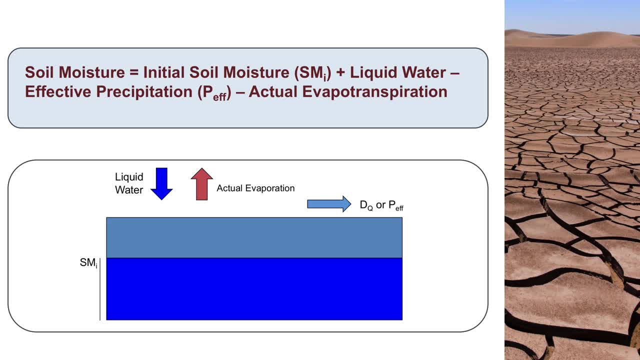 Initial value of soil moisture is given. We assumed 100. Liquid water: we have already calculated it. Also, effective precipitation and actual evapotranspiration are now in our Excel spreadsheet. Now we can move on to calculating soil moisture. Now we can move on to calculating soil moisture. 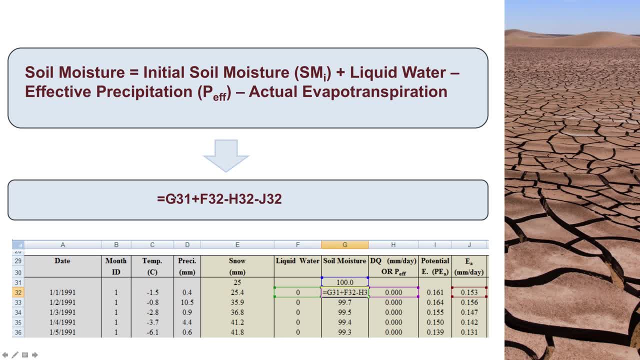 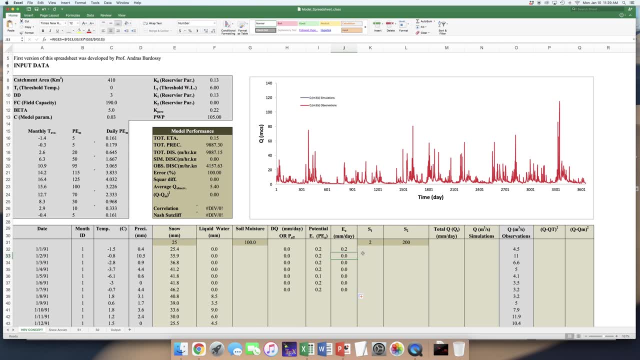 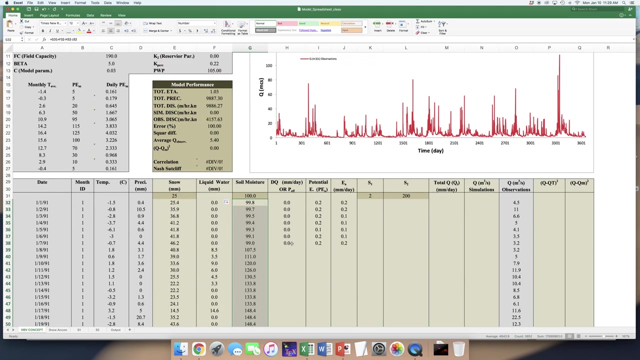 calculating soil moisture. Here is the equation Back to soil moisture. As you can see here. these are the variables we are using. They are highlighted here. Now we have updated soil moisture: direct runoff or effective precipitation and actual evapotranspiration. 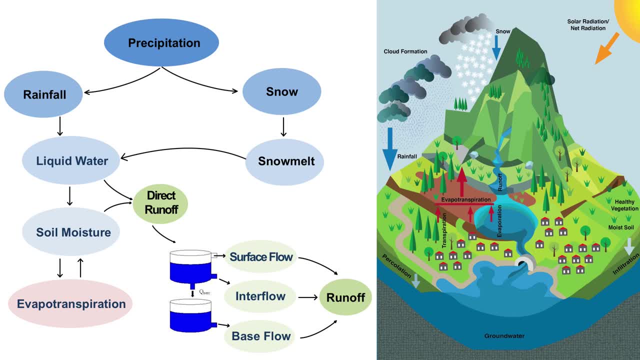 So back to our model structure Now. the next step is to calculate runoff. Here we use a bucket model concept. It is widely used in conceptual hydrologic modeling. Depending on your study area and data you have, you may go with one bucket or two buckets. 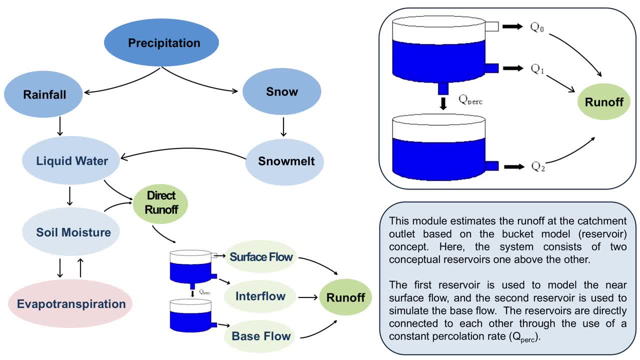 or even more. Here we go with two buckets describing near-surface and subsurface processes. We want to simulate surface flow interflow and base flow contributions to the overall runoff. Again for definitions of these terms, review hydrology textbooks. 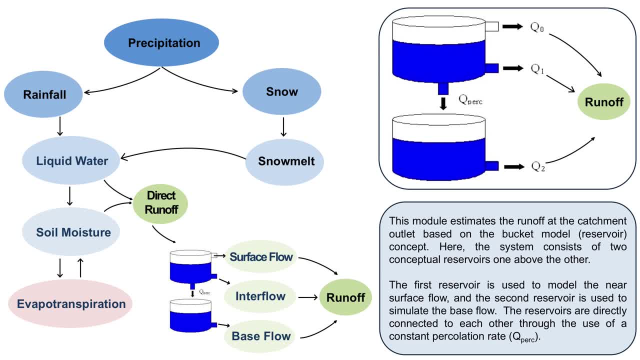 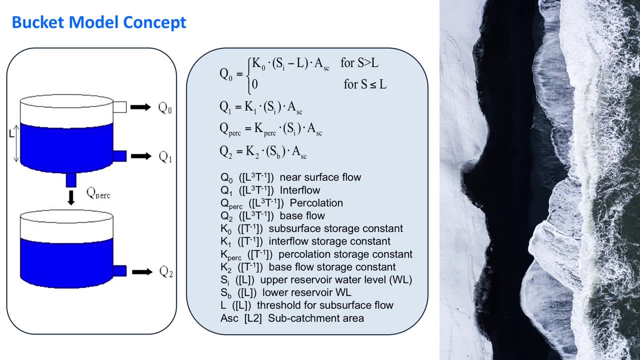 In this lecture we focus on modeling these processes. Here are the equations we use for estimating outflows from these two buckets. Here we have four discharge values. One connects the two together, that's Q percolation, And the other three contribute to overall runoff. 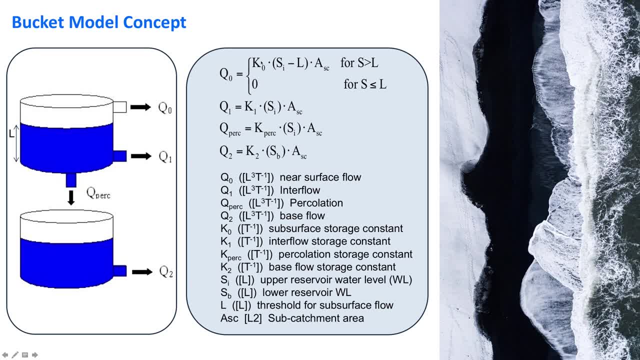 The equations are linear. Each one has a parameter k. It's called storage constant or reservoir constant. It has a unit of inverse time. Outflow is a function of s or storage. If there is no storage, there is no water. Basically, we assume there is no contribution to runoff. 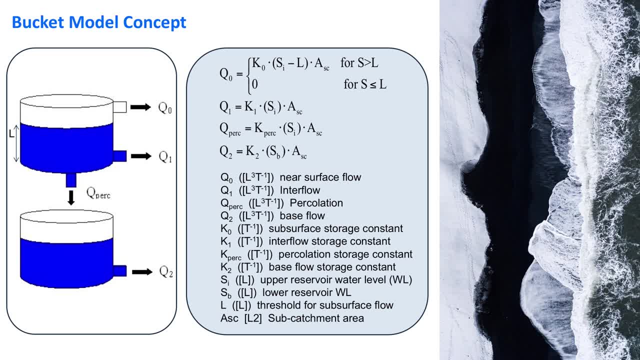 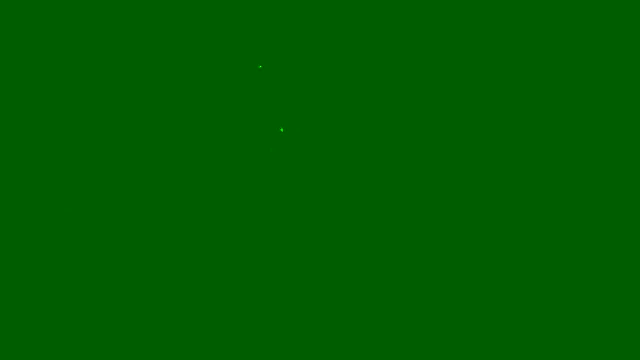 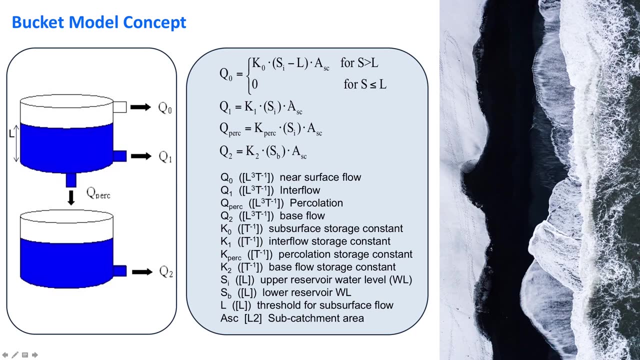 But if there is water, some of that contributes to overall runoff. Here uppercase Q represents volume, K times s, times A. A is area of the watershed. If we remove A, then we will calculate Q in unit length. That's what we do. 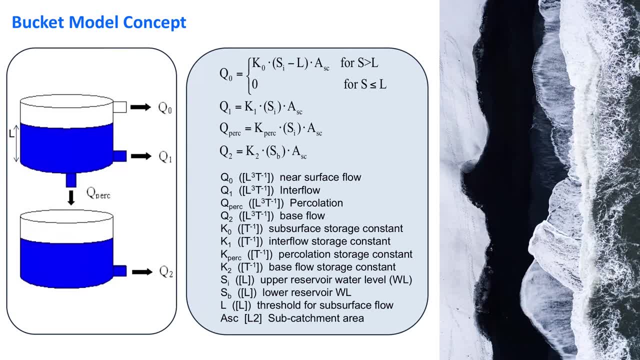 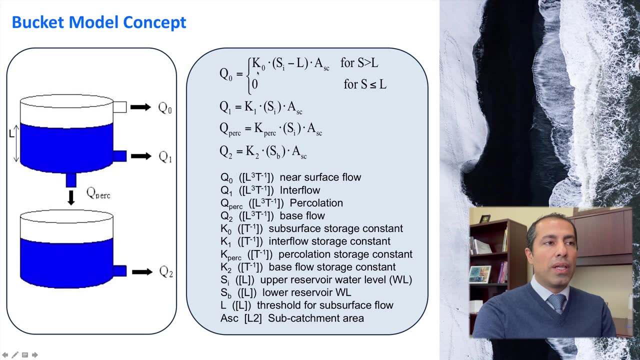 In our Excel spreadsheet, because so far we have used unit length. we calculate lowercase q or Q in length unit And then later toward the end we multiply by area to calculate volume Q naught, or the first outflow is a bit different than the other ones. 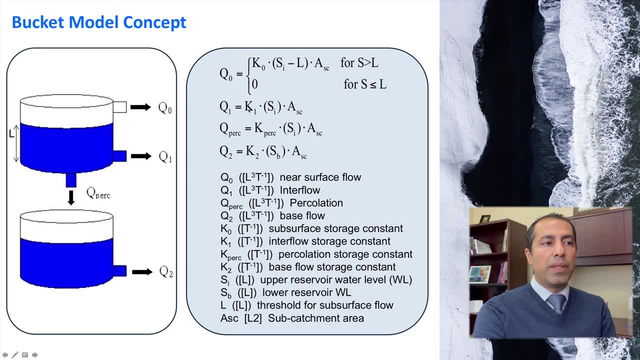 Q1, Q percolation and Q2 are simply k parameter times s storage of that bucket. Q1 and Q percolation: Q percolation are a function of s1, or storage of the upper reservoir, And Q2 outflow is a function of sb, or storage of the second reservoir or baseflow reservoir. 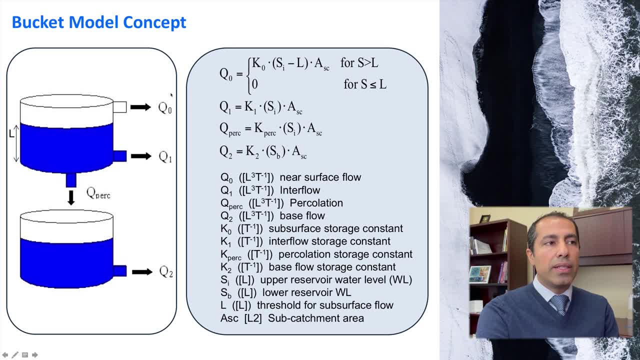 The first one. the outflow is at the very top. It is designed to describe fast and immediate contribution to runoff. First we need a threshold, L. We assume that if a storage is below L there is no outflow from the top of the bucket. 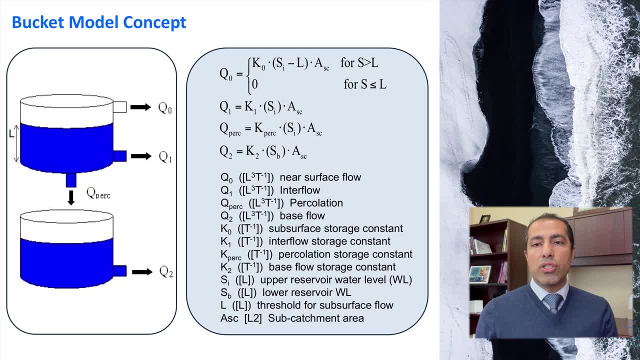 It means there is some room for storage and water remains in the basin for a while until it reaches a threshold, and then it starts contributing to runoff. If storage is above L, then again we have a similar equation. The difference is s, or storage level in the upper reservoir or upper bucket, minus our threshold L. 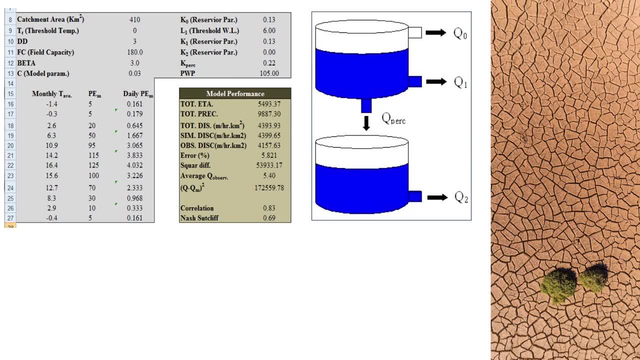 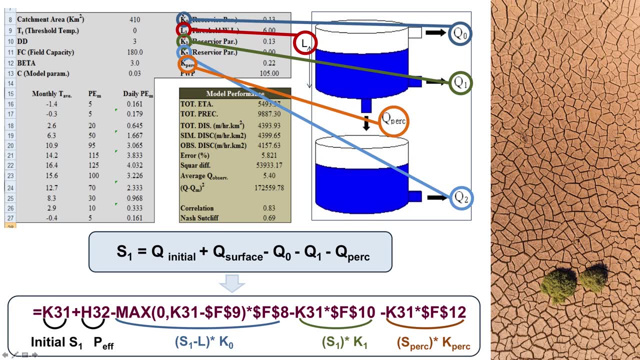 L times K0.. So we need to add new parameters to calculate storage and later runoff. Here are the parameters we use in our Excel spreadsheet: K0 for Q0.. K1 corresponds to the bottom outflow from the upper bucket. L is storage threshold. 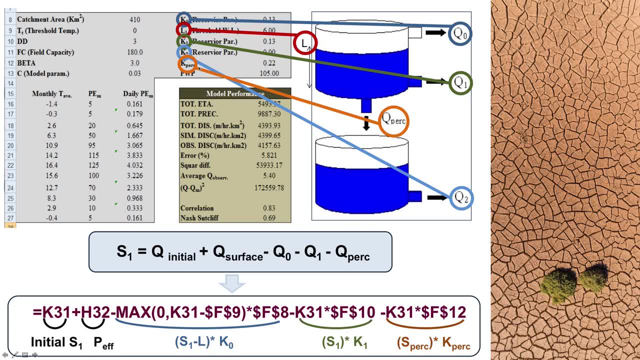 K2 is for Q2. And K percolation represents the connection between the two buckets. Where do we get these parameters? Again, we make an assumption And then later we estimate these parameters and double check our assumptions, Since outflows are functions of s values. 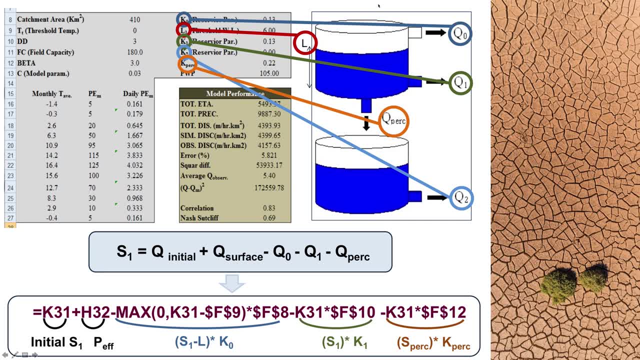 we need to calculate storage S1 for the first reservoir and S2 for the bottom reservoir. Our general equation is like this: Storage of the upper one is equal to initial value of storage. We always assume there is some initial storage plus inflow to the system, minus the three outflows. 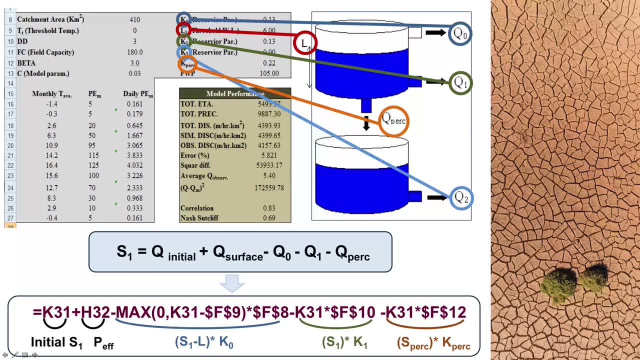 Minus Q0, minus Q1, minus Q. percolation: Initial value in our Excel spreadsheet is 2 mm And Q surface is what you have calculated before as direct runoff or effective precipitation. In our Excel spreadsheet we use unit length. 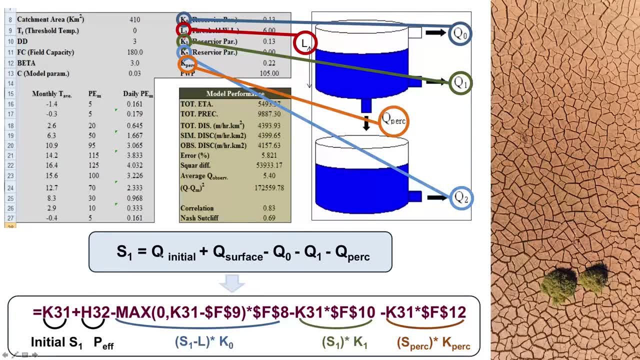 So storage in length and Q also in length. So for now we don't multiply by area. We will take care of area at the very end. So this is our equation: Initial value of storage plus effective precipitation or direct runoff, minus first Q0, minus Q1, minus Q2.. 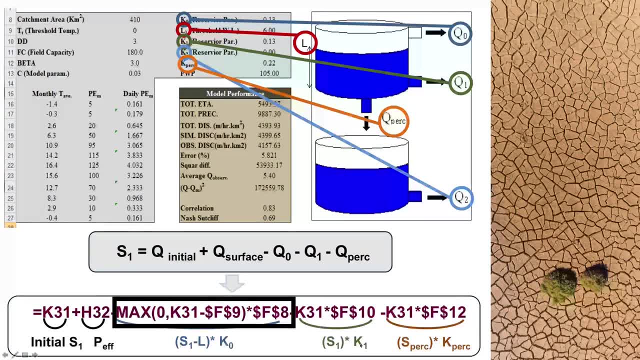 These two equations are very simple: S times K For S, we are calculating S1.. But we also need storage to calculate these two terms, So we use the initial value of storage For the first one. again, it's a two-part equation. 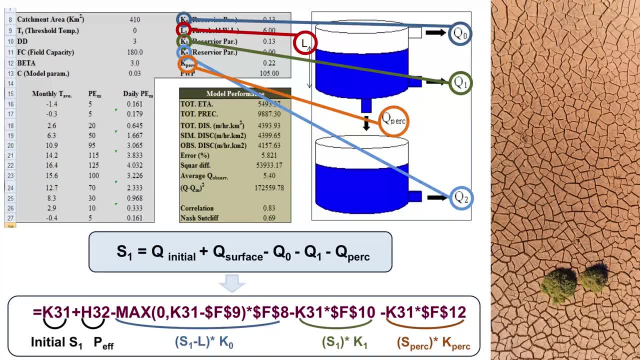 If storage is less than L, then there is no storage, Then there is no outflow, There is no Q0.. So use the maximum of 0 and this term S minus L times K0. Let's do that in our Excel spreadsheet. 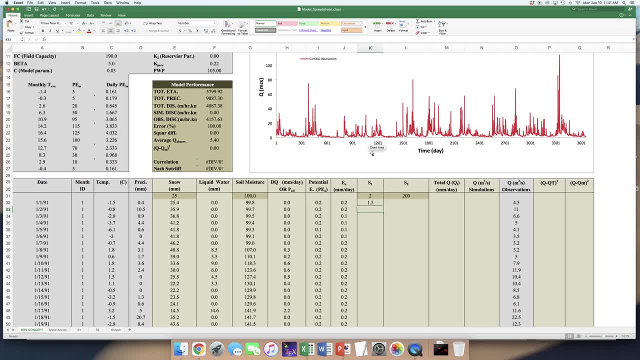 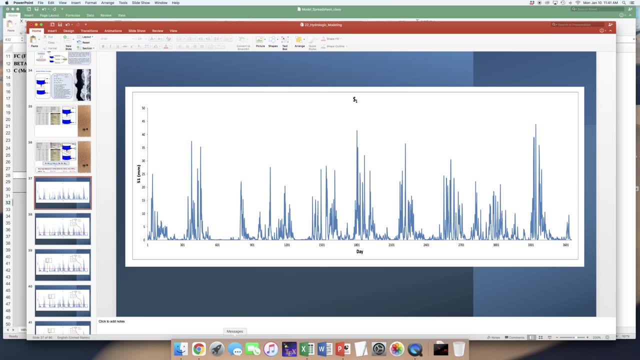 Again, the initial value is something you assume, But later we will revisit our assumptions. Here is S1.. This is what we just calculated. You can see that in the Excel spreadsheet It appears in one of the tabs. What we have calculated is storage in millimeter. 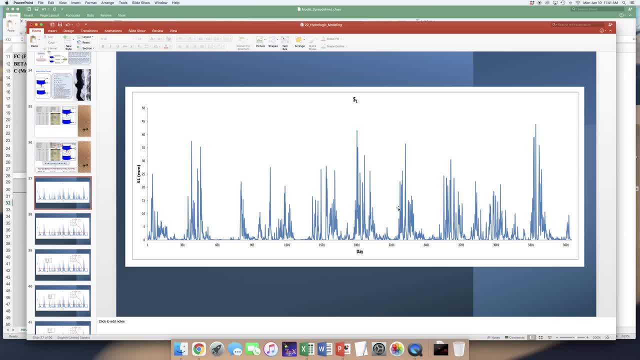 So unit length. You can see it's a highly variable Time series Because we are looking at a relatively shallow depth of soil, So it's near surface And there is high variability. Let's assume that in our equation L length is 10.. 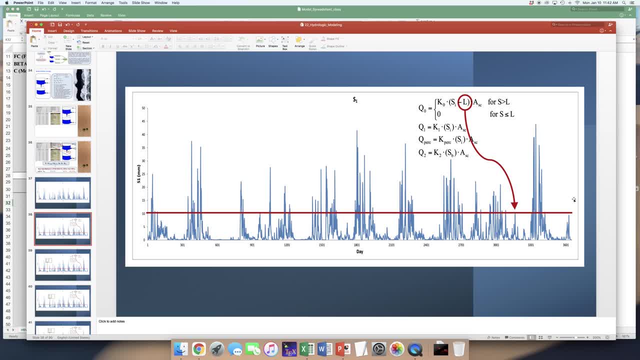 So I'm drawing this horizontal red line as my threshold. Let's assume this is what we used to calculate S values. If I'm here on the X axis, It means there is no storage, So no Q0.. Q0 will be 0. 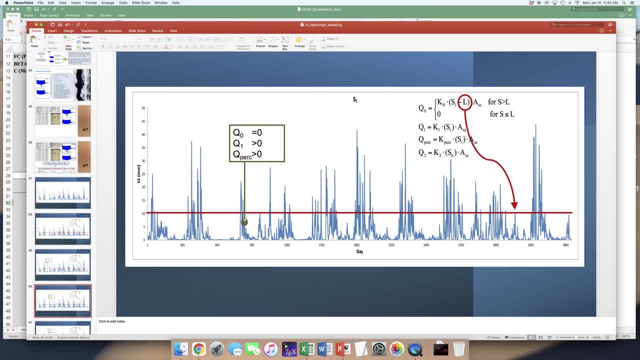 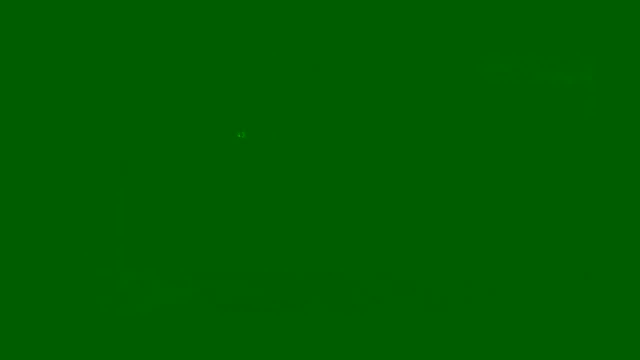 Q1: 0.. If I'm looking at a value between 0 and the red line, So here, for example, S equal to 5.. Again, Q0 will be 0, because 5 is below my red threshold. So Q0 will be 0.. 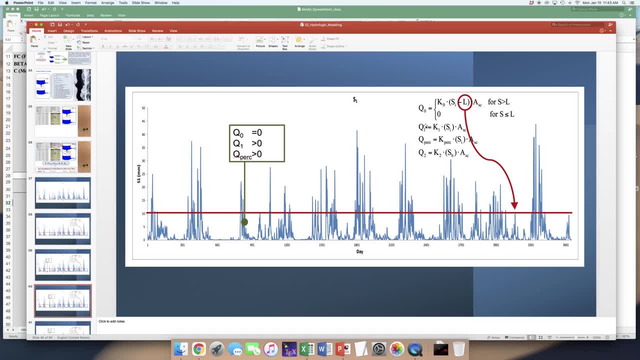 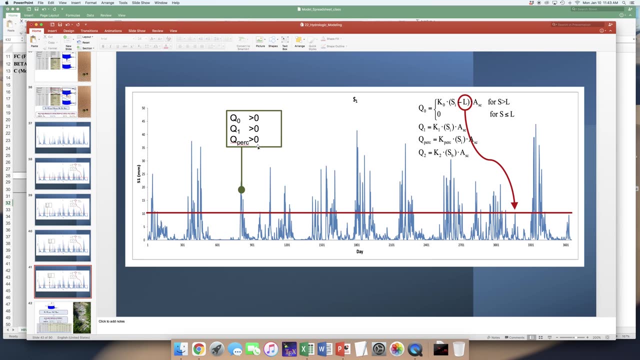 But I have non-zero Q1 and Q percolation. If S is larger than the threshold, Then all three values will be non-zero And they all contribute to the overall runoff. K percolation goes indirectly through the second reservoir. Now let's look at the second reservoir or the second bucket. 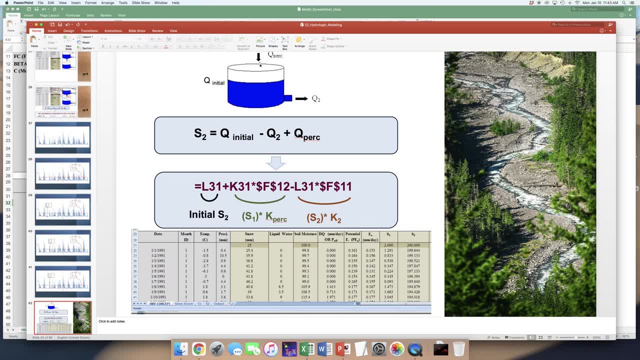 Here we have one inflow, That's Q percolation, And one outflow, Q2.. Again, we assume an initial value, So S2 is equal to Q initial Minus Q2 plus Q percolation. Again, we are calculating S in unit length. 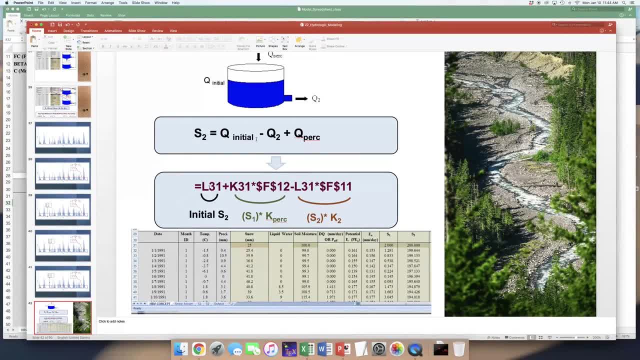 So for now we do not multiply by area. Initial value of S2.. L31 plus S1 times K, percolation Minus S2 times K2.. Here the initial value of S2 is 200.. As you can see, we use larger value for S2 relative to S1. 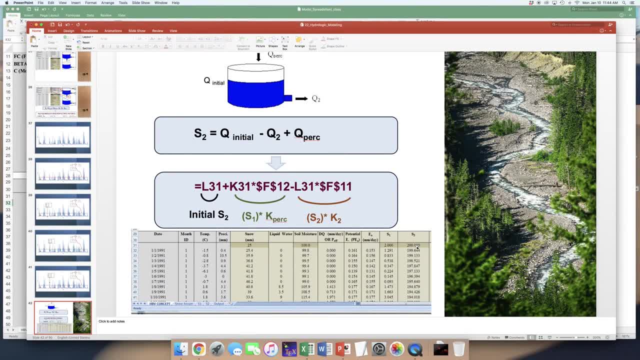 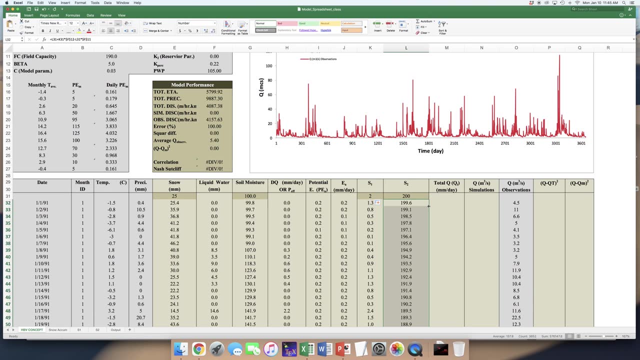 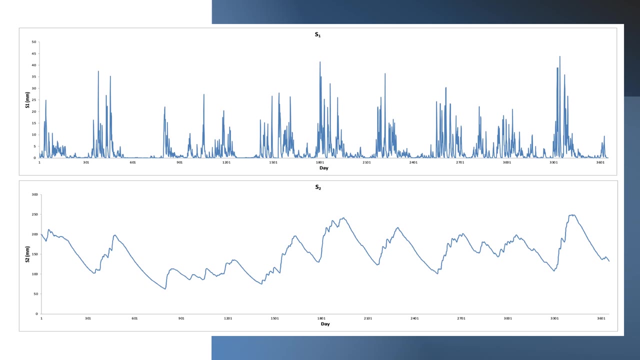 Because here you're using the first bucket for near surface shallow processes And S2 is groundwater base flow contribution to runoff. Now we have S1 and S2.. Let's look at S1 and S2 together. There is a big difference between these two. 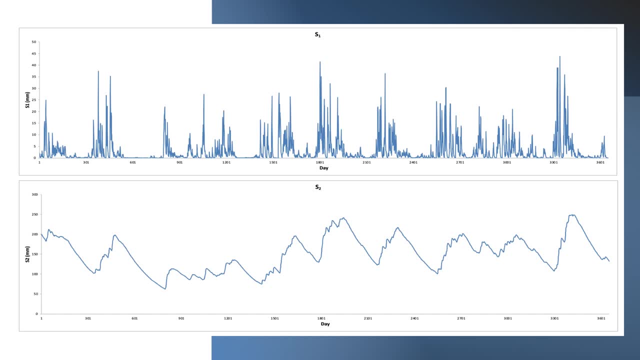 As you can see, S1 is highly variable. S2 is less variable, Changes slowly. We use very different initial values. The second one changes really slowly Because, you can imagine, groundwater responds really slowly to changes in precipitation. To do that we have to make sure our parameters are reasonable. 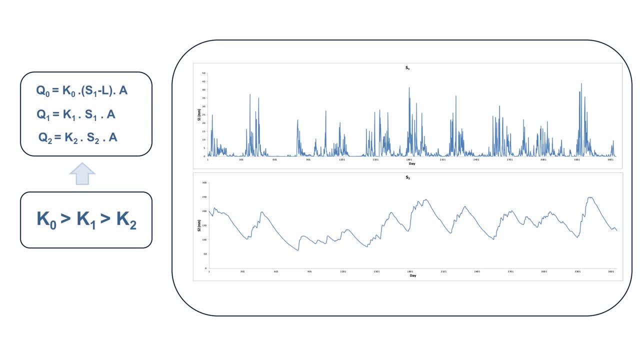 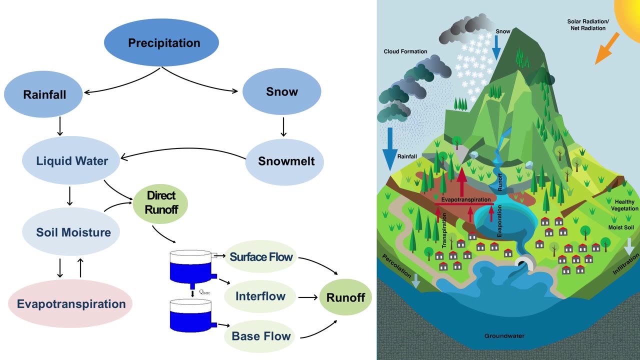 We do that through K values. K has inverse time unit, So to make sure we get something like this: K0 should be larger than K1.. K1 larger than K2.. Back to our model structure. We calculated the outflows from our bucket models. 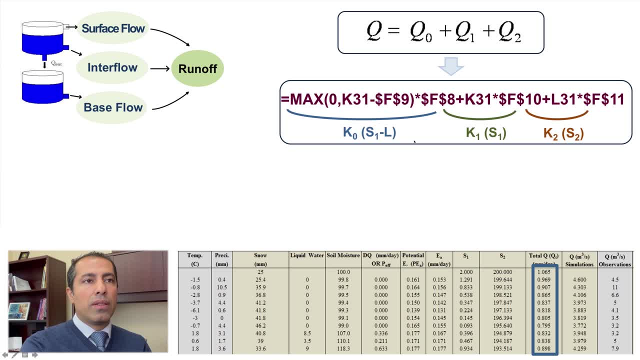 And now we are ready to calculate runoff. Here we assume runoff is simply Q0 plus Q1 plus Q2.. The three outflows from our bucket models. Here is the equation for Q0 plus Q1 plus Q2.. Again, K times S for Q1 and Q2.. 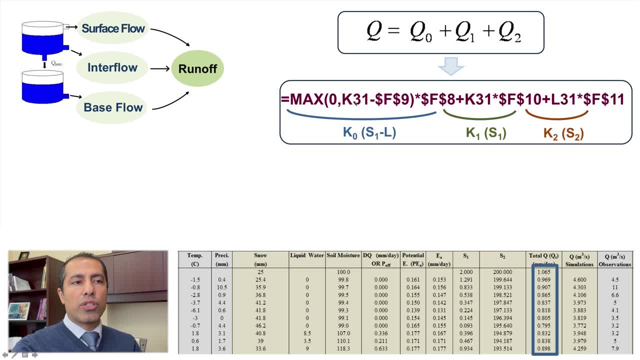 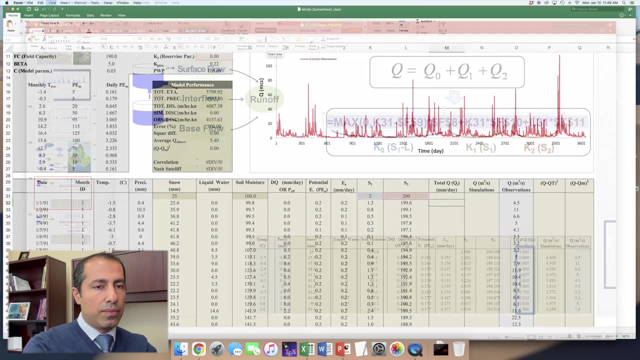 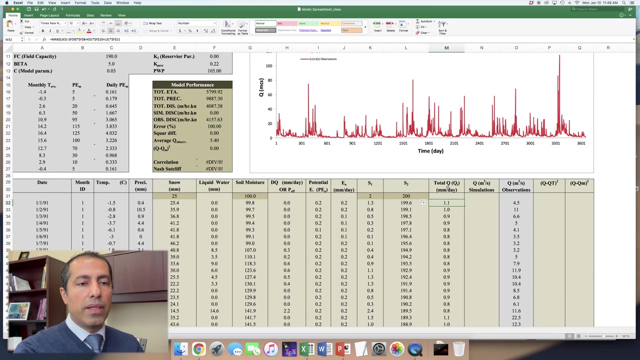 For the first one, we use a maximum function: S1 minus L. If this term is negative, then there is no Q0.. There is no contribution from Q0.. The output is still in unit length, As you can see here. 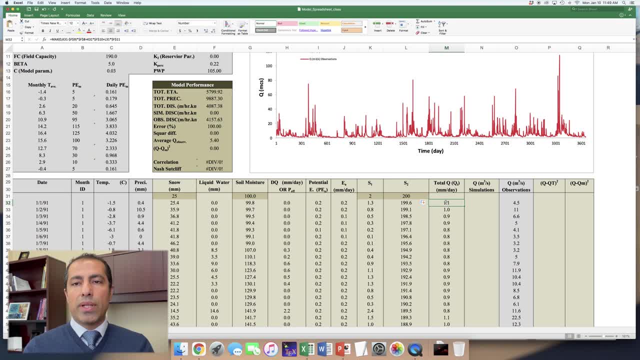 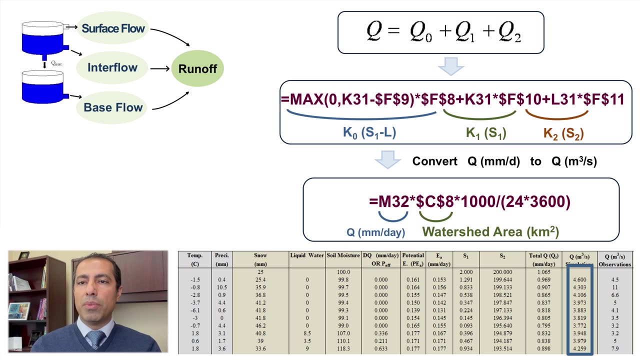 So it's millimeter per day. Now that we have calculated the overall Q, Now we can multiply by area and calculate the volume of flow Like meter cube per second. This is how we convert from millimeter per day to meter cube per second. 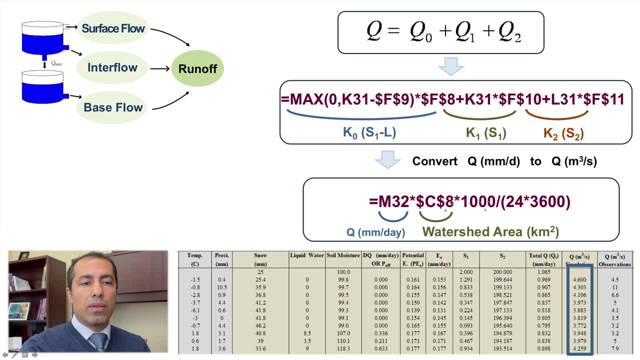 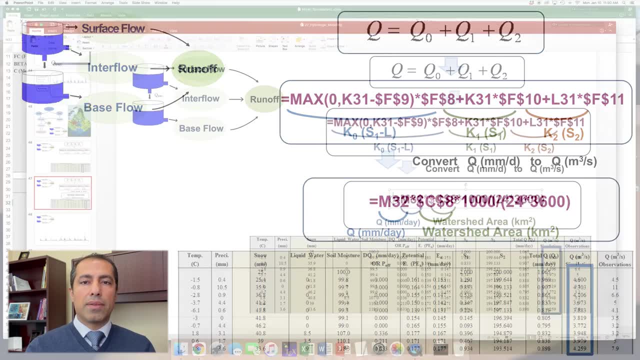 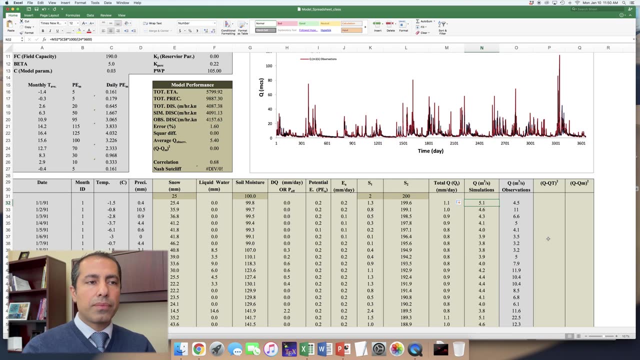 We multiply by area And we do unit length And we change So that we calculate discharge in meter cube per second. We just calculated runoff And we also have some real observations from our study area. The gray column here Next to our simulated runoff. 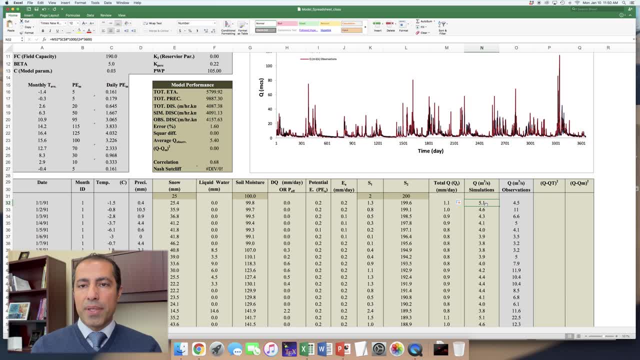 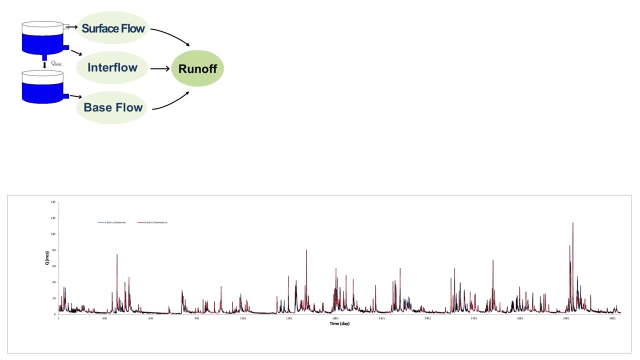 Called it Q observations. These are real observations. We are going to evaluate our model against observations And revisit our parameters and initial values. The Excel spreadsheet gives you simulations and observations next to each other. As you can see, The two are pretty consistent. 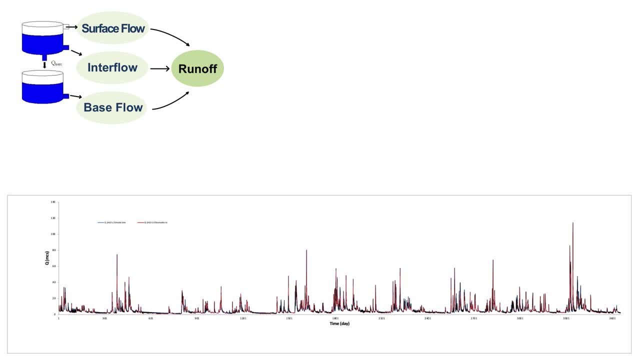 Because I used very reasonable parameters. In reality, when you do this for the first time, Simulations and observations may not look similar, But there are ways to adjust and calibrate your model. If we zoom into this part of the graph, You can see that the peaks are simulated reasonably well. 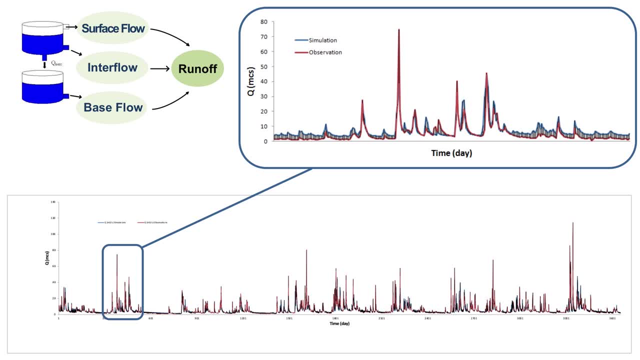 But there are biases in low flows. You can see that simulations in low flows are systematically higher than observations. If your objective is simulating peak flows, This is probably already good enough, But if you also care about low flows And you want to make sure they are reasonable, 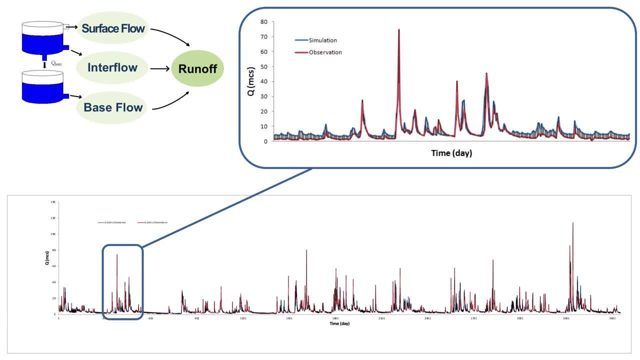 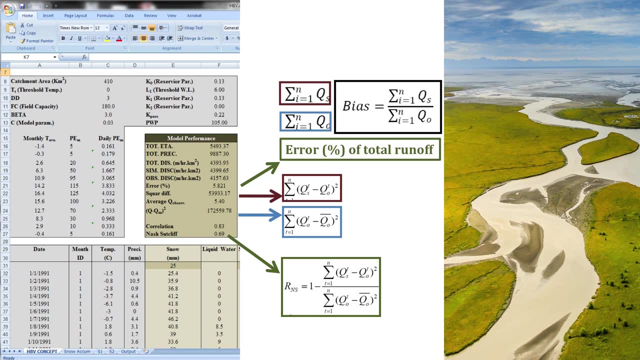 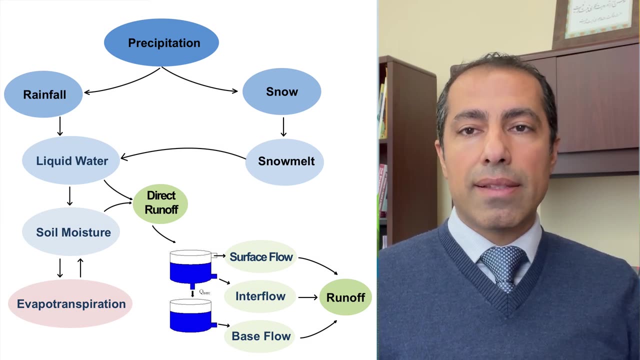 You have to go back and adjust our model parameters In our Excel spreadsheet. There are some metrics there That we will use to evaluate our model And later estimate our parameters. So far we have calculated runoff And in the next lecture We will talk about model parameters. 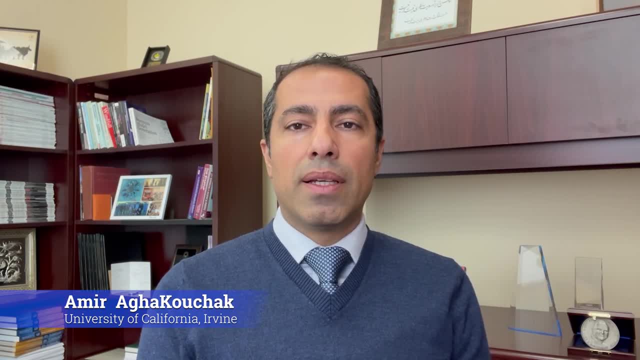 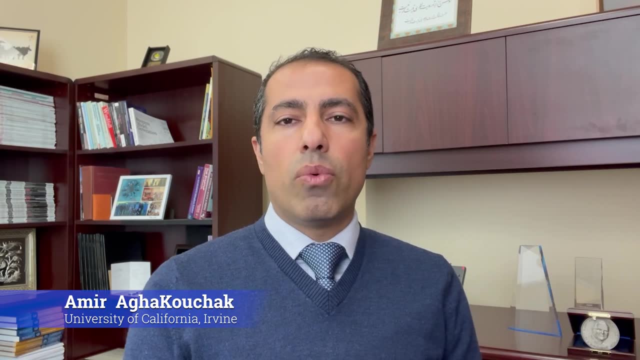 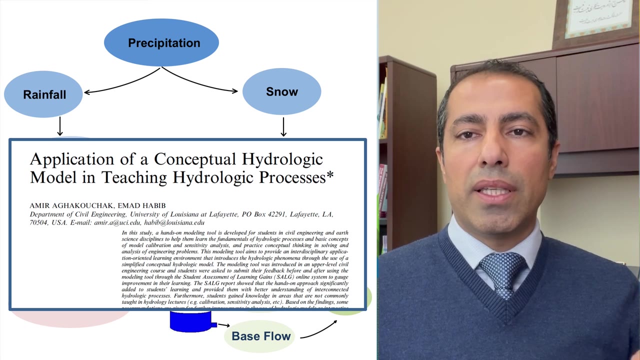 How to check the assumptions we make, Update parameters And optimize our model To make sure simulations are consistent with observations. The details of the model I presented Are available in this paper, Including the equations, And you can find some additional references. 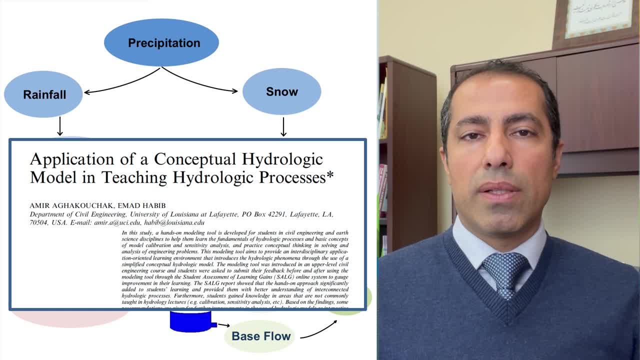 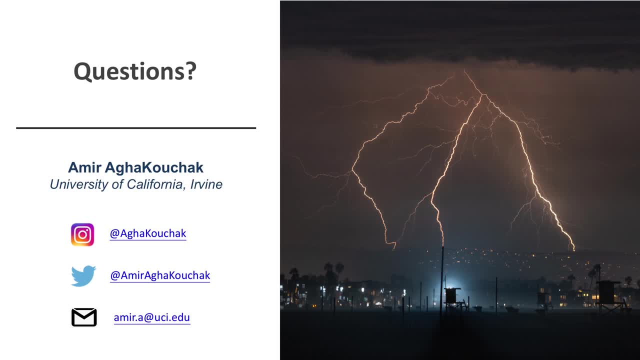 To the original publications on this model. Now continue to the second part, So that we can update our model parameters. If you have any questions, Feel free to contact me Or add your questions in the comments. I will try to respond to all of them.